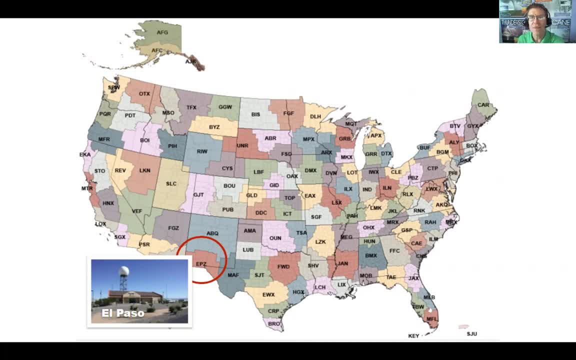 working in your local National Weather Service office that are issuing the warnings to let you know when the bad weather is coming to town, And that could be a flash flood warning, It could be a tornado warning, It could be a blizzard warning if you live someplace where you get blizzards. So 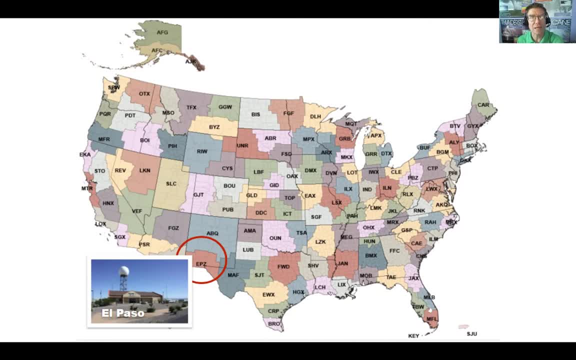 it's the mission of the National Weather Service to protect lives and property from the weather. Now, each of these weather offices also, in addition to issuing warnings, also issue weather forecasts. Now, weather forecast is simply a guess or a prediction of what the weather. 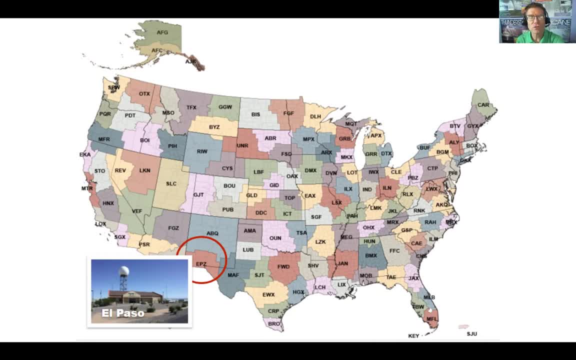 is going to be sometime in the future. That future can be five minutes from now or that future can be seven days from now. It just depends on which forecast we're issuing, because we issue different kinds of forecasts. We issue forecasts for pilots who fly the big planes that land at 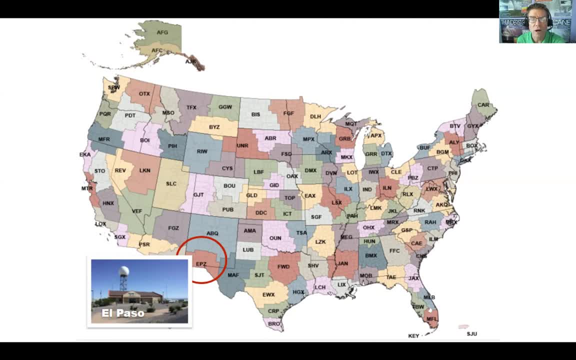 the big airports, but we also issue forecasts for some of the smaller airports, for the single engine planes. We also issue forecasts for boaters on any of the lakes, the rivers, the coastal borders of the United States. We issue forecasts for the men and women who fight the forest fires. 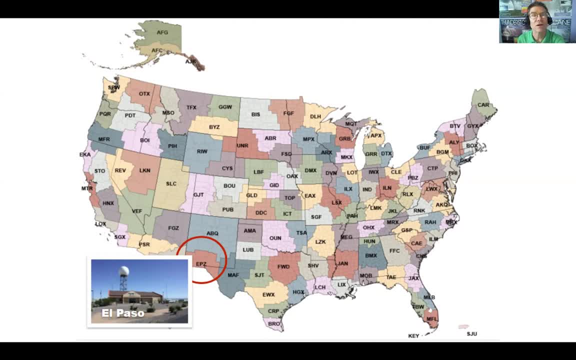 in the mountains and in the grassland fires down in the lowlands, And we also issue forecasts for people like me and you, and that includes things- and we call that the public forecast- which includes things like: is it going to be hot, Is it going to be cold, Is it going to be rainy, Is it? 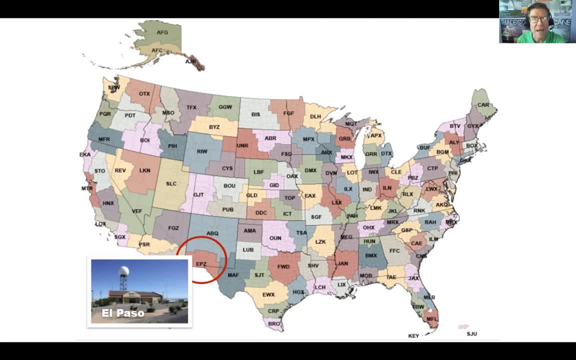 going to be snowy? Is it going to be sunny, cloudy, windy, calm, anything like that, so that you can decide whether you need to. you know if you need to take an umbrella, if you're going to the grocery store, whether you need a weather jacket if you're going out to the grocery store, whether you need a. 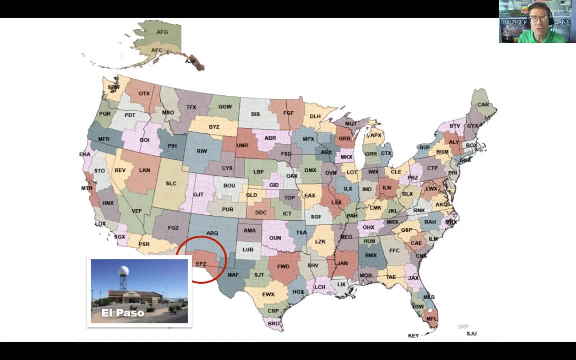 side? or can you wear shorts if you're going to go out to play Again? the mission for the National Weather Service is to protect lives and property from the weather and to help people make wise weather decisions. And you know what People ask me all the time when: where does the weather come? 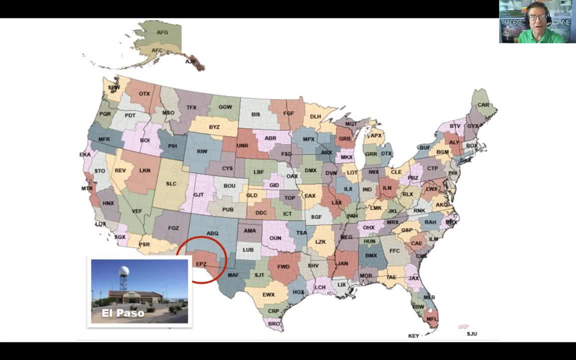 from. And I wish I could say we had a big machine where we just pushed a button and you know, we could say, make it sunny today, make it cloudy today. but it just doesn't work that way. We don't have any control of the weather. but we do have a good way of forecasting it. But you have to. 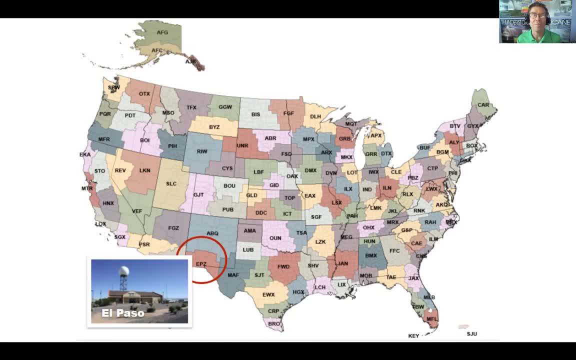 understand where the weather is coming from, And I think that's a good way of forecasting it. You have to understand where the weather starts to understand how to forecast it. And on the earth, where the weather starts, it all starts with the sun, So we have to get off the earth. 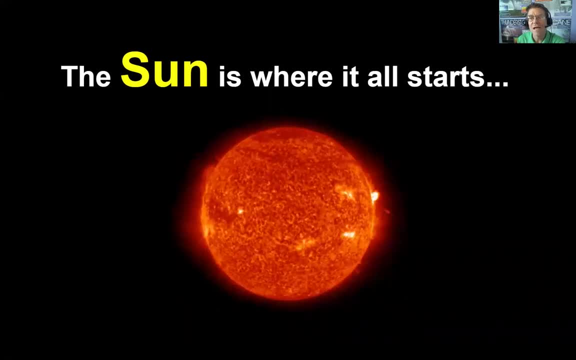 and look to that big glowing gas ball up in the sky to see where all the weather starts on the earth. The sun, as you know, is super duper hot and it is what starts all the weather on the earth. That sunlight heats up the earth. If you've ever gone outside on a summer day, you felt that. 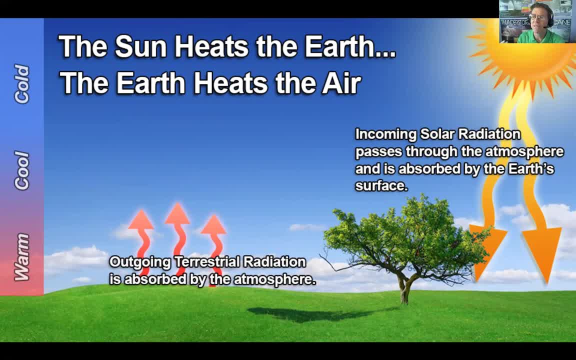 sun shining on your skin. You can feel how warm that is. Well, the sunlight passes through the air, heats up the ground and then the ground starts to heat up the air from below. A lot of people think that the sunlight is heating up the air, but it actually passes. 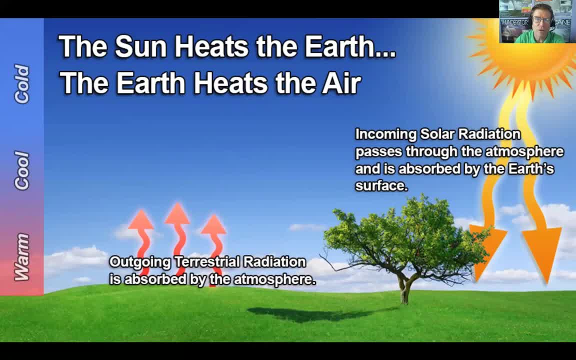 through the air, just like the light shines through a window. And then that light strikes the ground and it starts to heat up the ground and the ground warms up from you know, the ground starts to warm up the earth from below. It's the same concept. If you've ever seen mom or dad put 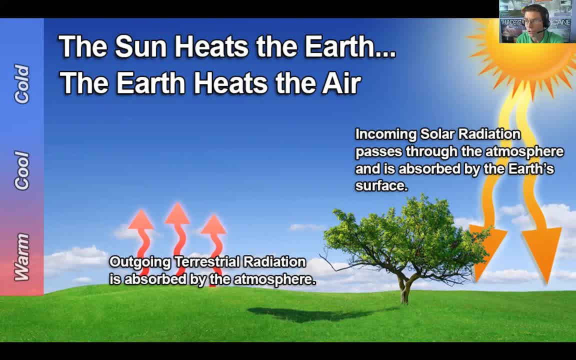 a pot on the stove and they've turned that burner on, that burner starts to heat that pot up from below. So if you've ever- you know, if you've ever- got up in a plane, you, it's nice and comfortable inside. 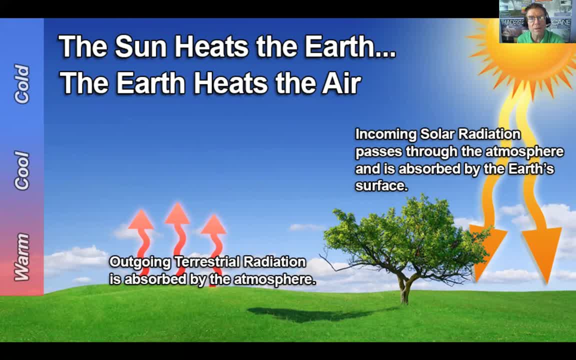 the plane but, believe it or not, right outside that window it's super duper cold because as you move higher up into the atmosphere in general it gets colder, as it kind of shows here. It's warm near the surface of the earth and cooler and colder, And you've seen this, if you've ever. 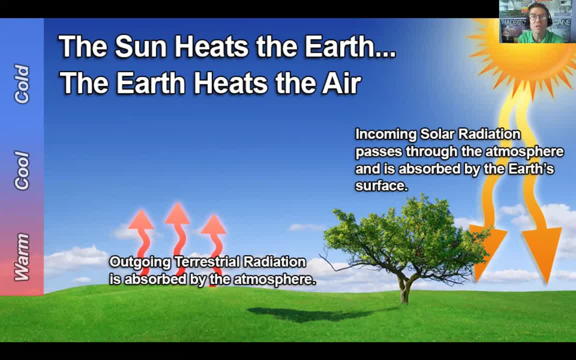 been to the mountains, you know, as you go up into the mountains usually it gets colder as you go up into those mountains. So again that sunlight passes through, the air strikes, the ground starts to warm up the ground and then the ground warms up the air from below. So as you move up away from 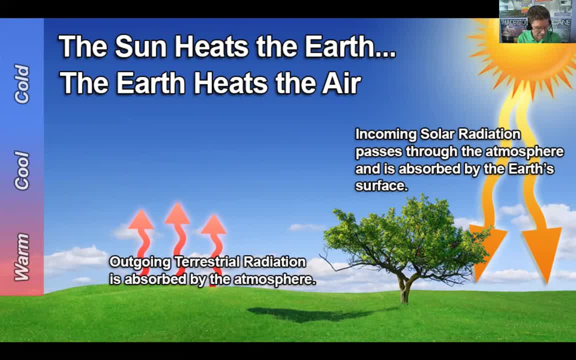 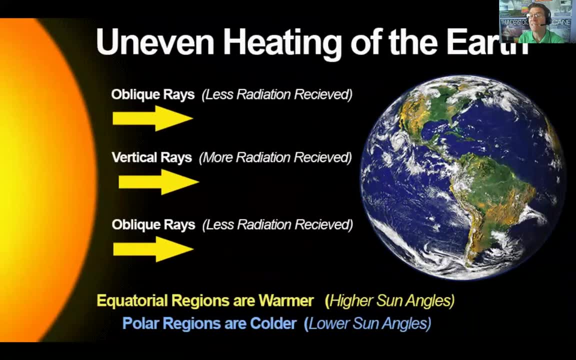 the ground. it's going to get cooler because you're moving away from what's warming up the air. All right, we're going to talk about three interesting facts about the earth. Interesting fact number one about the earth is it is round. We live on a big beach ball, but because it's round, 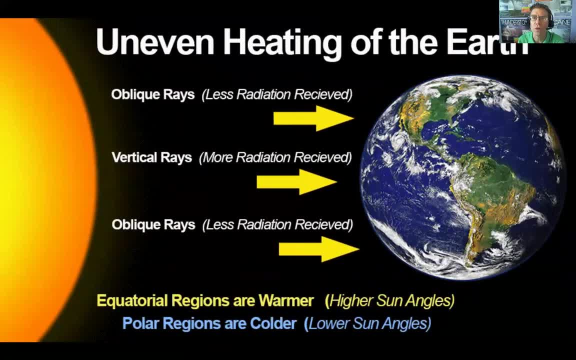 the sunlight coming from the sun does not strike the earth evenly because it's curved. The earth has got this curvature on it. You can see these arrows kind of represent the sunlight. You can see how in your mind, you can see how the sunlight is striking more directly in the middle part of the earth versus as you head. 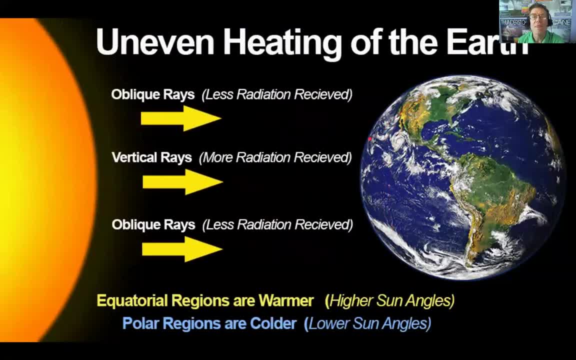 up towards the north or south poles, the top or bottom of the earth, the sunlight gets spread out over a wider area because that earth is kind of curving away. It's the same concept. if you ever take like a flashlight and you hold it straight up and down over a desk or a table, you can see it. 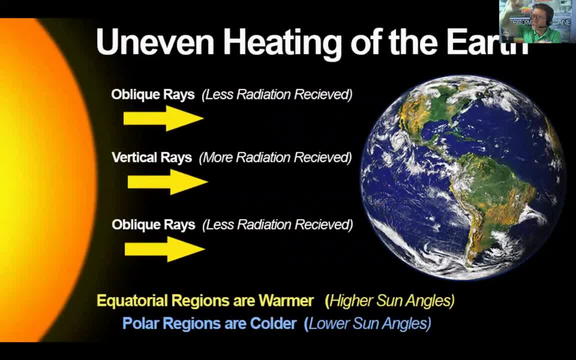 makes that concentrated circle right there on that circle. But if you start to tilt that flashlight you can see that the sunlight or the light from the flashlight I should say it's the same amount of light but it's spread out over a wider area and it's dimmer. The same thing is happening on 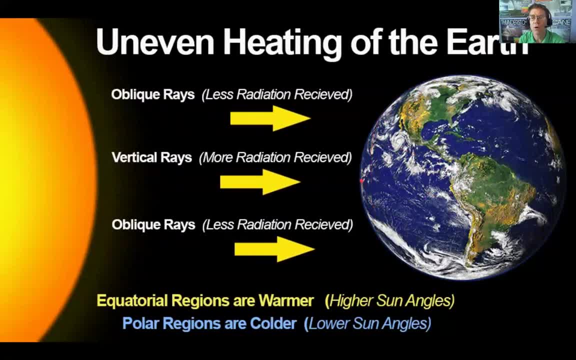 the earth As you move up towards the north or down towards the south pole. that light is being spread out over a wider area, so it's not as efficient in warming up the ground And because of that the north and south poles are colder than the middle part of the earth. I got another. 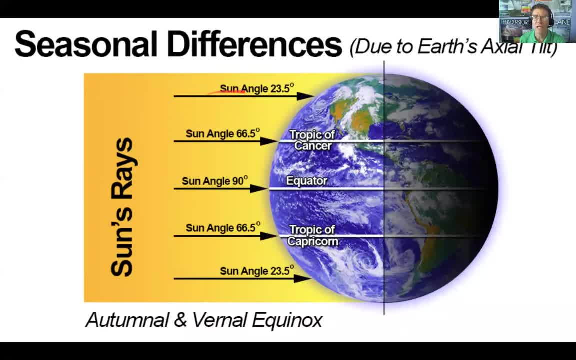 graphic here that might help explain it. The earth looks like on the first day of fall or the first day of spring. We even have some funny words down here: the autumnal and vernal equinox. Those are just funny. I shouldn't say funny Those. 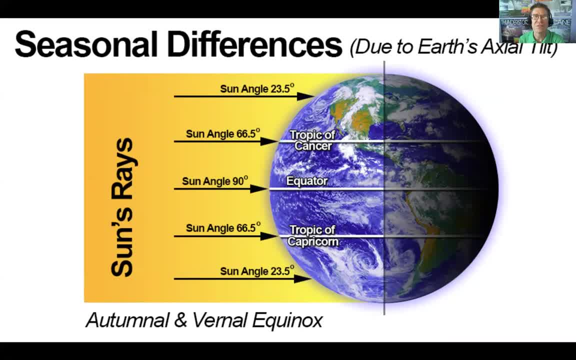 are just scientific ways of saying the first day of fall and the first day of spring. As a matter of fact, in the word equinox there you can hear the word equal, kind of hiding it. because roughly on the first day of fall and the first day of spring, your nighttime and your daylight are 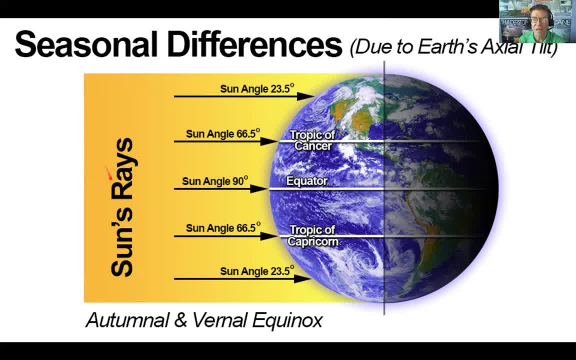 about evening. Well, anyway, on the first day of fall and the first day of spring, that sunlight's coming straight into the middle part of the earth. you know the equator. The equator is an invisible line on the earth, kind of like the belt of the earth. It goes right around it. This 90. 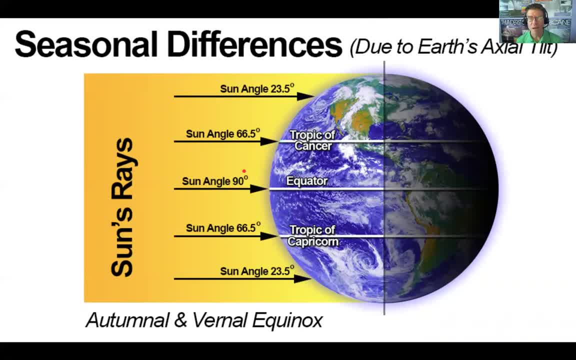 degree angle. I'm not talking about like 90 degrees temperature-wise, I'm talking about 90 degrees. when you're talking about angles, So you're talking about protractors or angles or compass or something like that. So that's that perpendicular, That's that sunlight coming straight in, And then 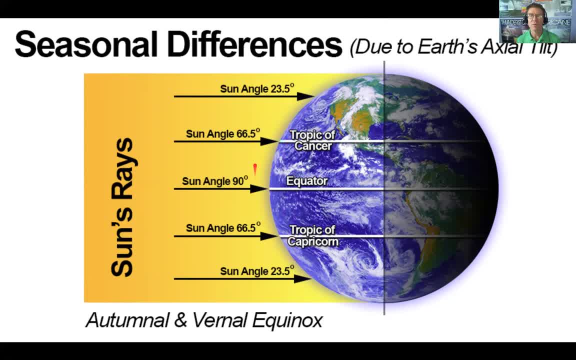 as you see, as you move up towards the north pole or down towards the south pole, that sun angle gets lower and lower. That's that same idea of tilting that flashlight more and more and that sunlight getting spread out over a wider and wider area. Now, interesting fact number two about the earth: 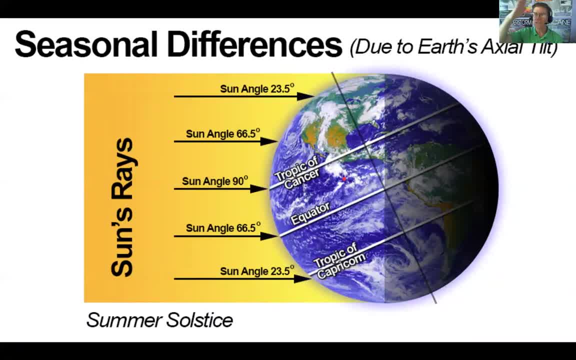 is that it is tilted. The earth actually leans over about 23 and a half degrees on its axis. Now we don't notice it because we're teeny-tiny compared to the earth And I don't want you to think the earth's going to like tip over or anything. That's just the way it is. It leans. 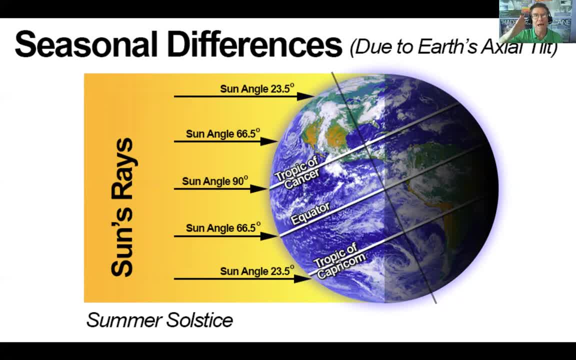 over like that. But because the earth does lean over on its axis, it leans over like that And that's what gives us our four seasons. This is what the earth looks like on the first day of fall, the summer solstice. Now you can see that 90-degree angle, that perpendicular sunlight. 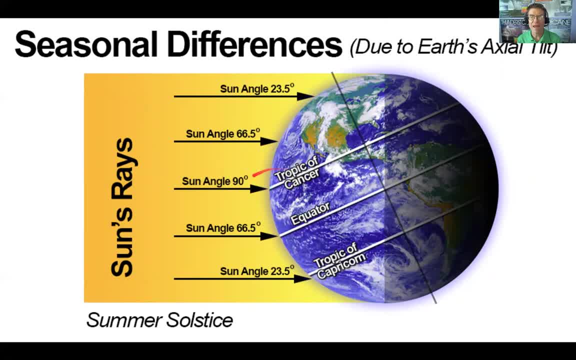 isn't coming in at the equator, It's coming in at the Tropic of Cancer. Now, Tropic of Cancer is just another one of those invisible lines. I don't know why they call it the Tropic of Cancer, They just do. But you can see how the more direct sunlight is coming into the northern part of the. 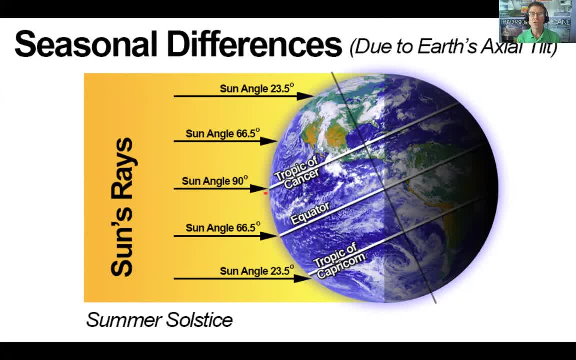 earth where we live. We live in what's called the northern hemisphere, So when the earth is part of the earth is kind of tilted over towards the sun, that's our summer. But guess what? The other bottom, the bottom part of the earth, the southern hemisphere, is actually kind of pointed. 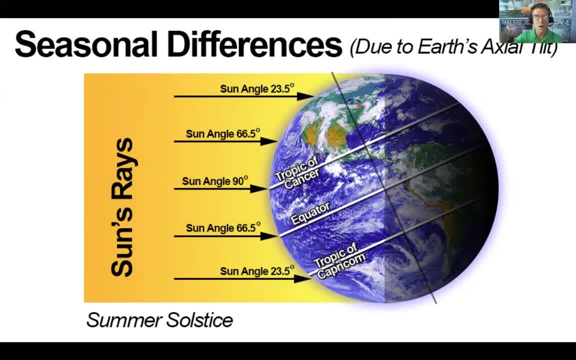 away from the sun, So that's their winter. So whichever part of the earth is tilted towards the sun, that's summer, And whichever part of the earth is pointed away from the sun, that's winter. So this kind of depicts you see that direct sunlight coming into the northern part of the 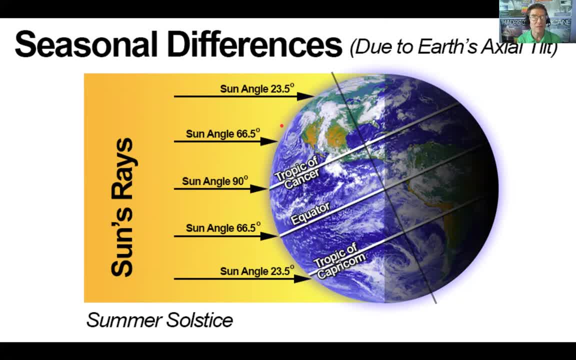 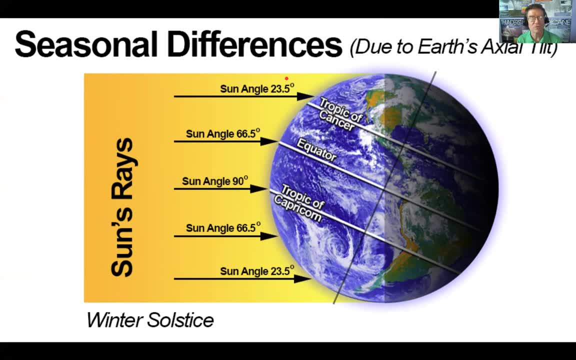 earth. So that's summer in the northern hemisphere where we live. But guess what, Six months later now the bottom part of the earth is kind of pointed towards the sun, And then top part of the earth, the northern hemisphere where we live, is tilted away from the sun. Now you can see that more direct. 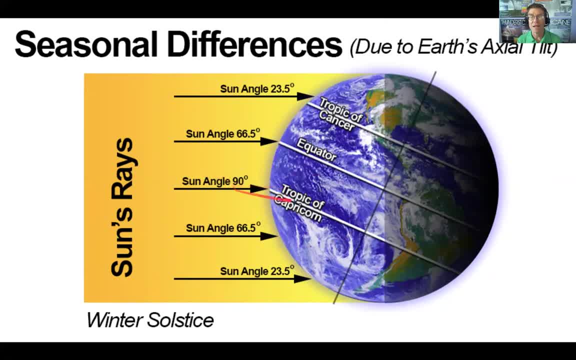 sunlight's coming into the bottom part of the earth And that 90 degree angle striking at the Tropic of Capricorn- Again, another one of those invisible lines on the map. So when it's winter in the northern hemisphere, where we live, it's actually summer in the southern hemisphere, And I 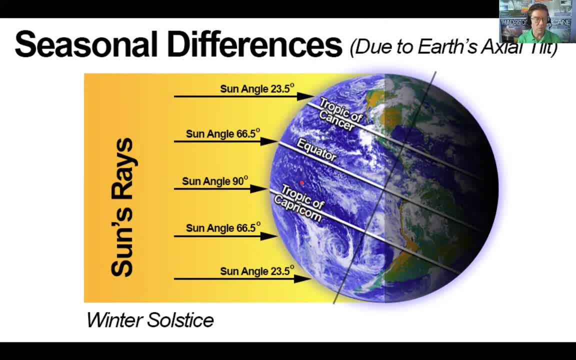 always think that's interesting. So you know when we're in the United States, when we're trying to figure out, you know what jacket to wear, what hat to wear and how many layers of clothes to wear because it's so cold outside. the kids down in Australia and New Zealand are trying to figure. 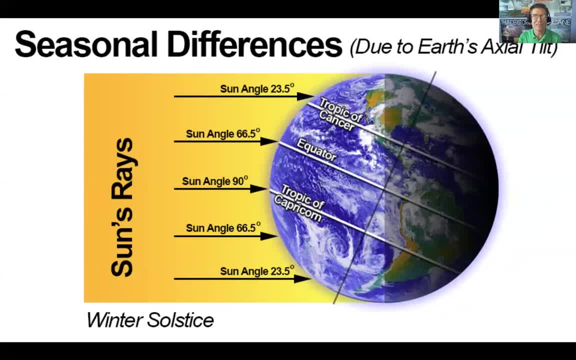 out which swimsuit to wear, which beach to go to and how much sunscreen to put on, because it's summer down there. So when it's winter in the northern hemisphere, it's actually summer in the southern hemisphere. Now I don't want you to think the earth is like wobbling back and forth, It's. 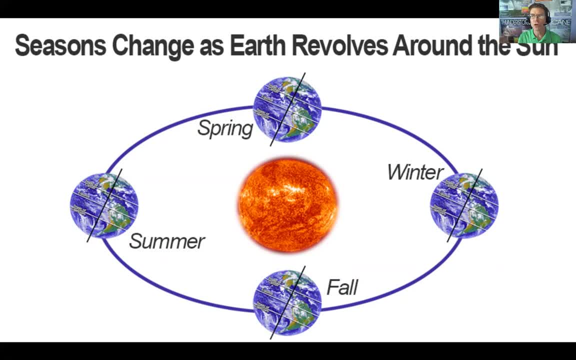 actually always tilted over in the same direction, But as we circle around the sun, or as we orbit, different parts of the earth are pointed towards and away from the sun. It takes 365 days to go around the sun. Of course that's one year. That's what makes one year. So if it's winter, you know. 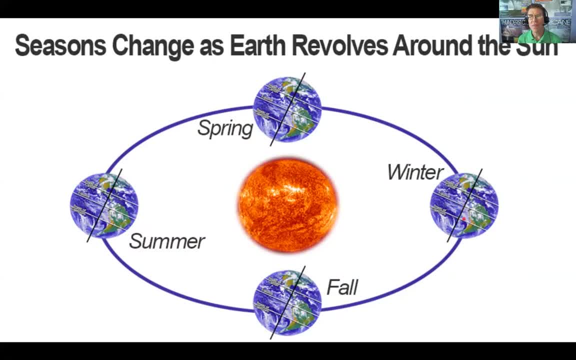 the top part of the earth is kind of tilted away from the sun and the bottom part of the earth is kind of tilted towards the sun. So you've got. you can see that it's winter in the northern hemisphere and then that means it's summer in the southern hemisphere. But look at this Six months. 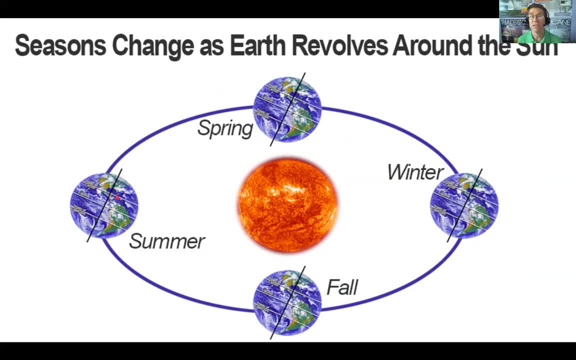 ago the earth was kind of tilted away from the sun. Now the northern part of the earth, the top part of the earth, is kind of tilted towards the sun and the bottom part of the earth is tilted away from the sun. So when it's summer in the northern hemisphere, it's also winter down there. 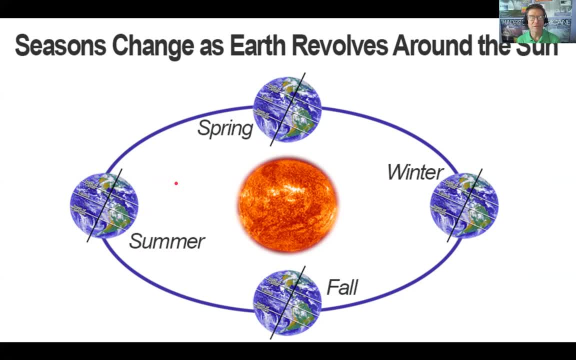 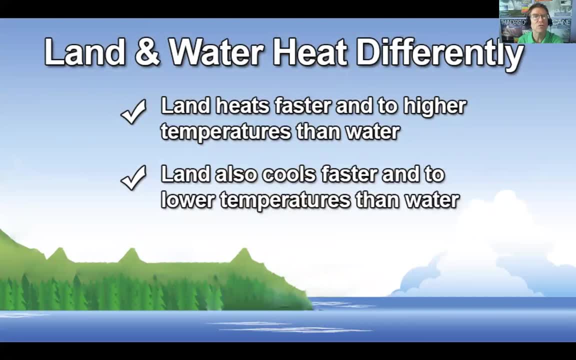 for the poor kangaroos and koala bears in Australia. All right. So interesting fact number one about the earth is that it's round. Interesting fact number two about the earth is that it's tilted. And interesting fact number three about the earth is that it's mostly covered with water. 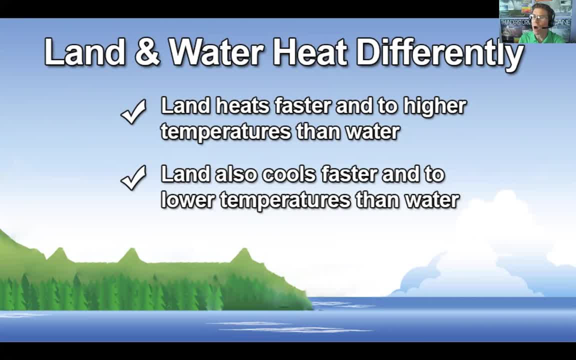 The surface is covered with water and land and water heat up differently. Land heats up fast, but it also cools down fast. Well, water heats up very slowly, but once water does heat up it holds on to that heat and is very slow to cool down. It's kind of like a heat battery. 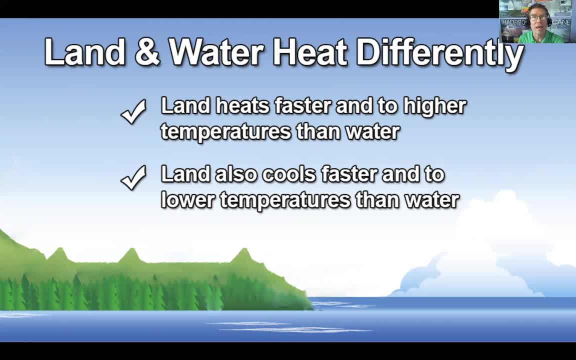 So a lot of times on the east coast and around the Great Lakes during the winter the land will kind of warm up during the day, but then at night it cools down. and it actually cools down so fast that it's cooler than some of the surrounding water that's near it. So it's very 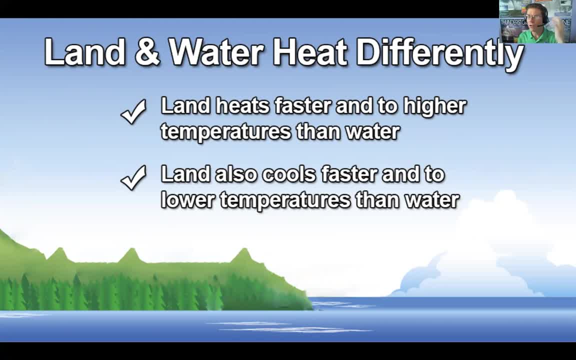 interesting. But we get this heating difference because land heats up very quickly And you may have experienced this if you've ever gone to the pool or to the beach or walking along next to the water, the kai, and your feet on that concrete or on the beach sand, it gets super duper hot, So you 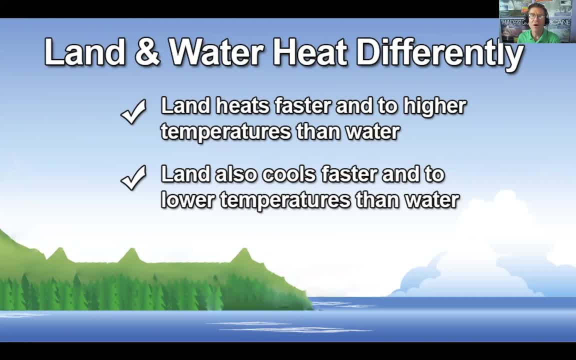 jump into the pool or you jump into the surf there and you go. ah, my feet feel much better. But if you think about it, the same sunlight is shining on the earth and the same sunlight is shining on the ground as on the water, but the water is so much cooler And, again, that's because 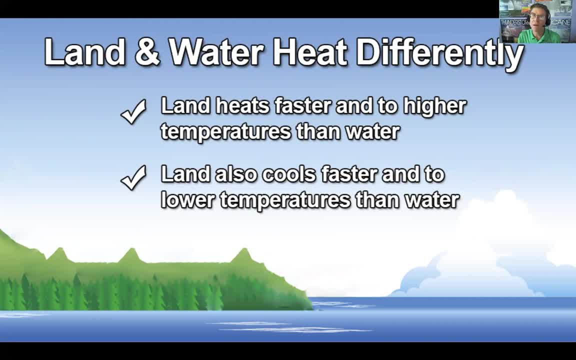 that land heats up quickly and the water takes much, much longer to heat up. But once that water does heat up, it actually holds on to that heat for quite a while- Now what we call this differential heating. this land heating up faster than water leads to some of the weather patterns. 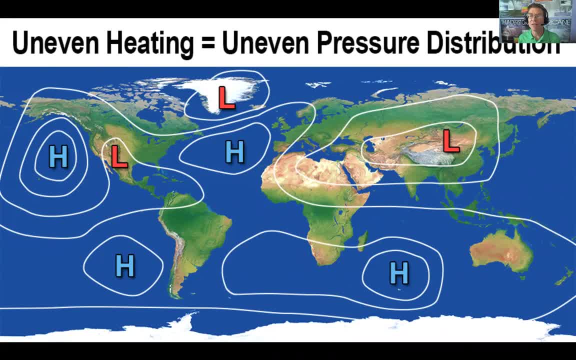 that we see This. uneven heating leads to uneven pressure distribution. Now, what is pressure distribution? All right, let's talk about that. If you've ever looked at the weather pattern, you may have seen some letters on there, some Hs and some Ls. The Hs stand for high pressure. 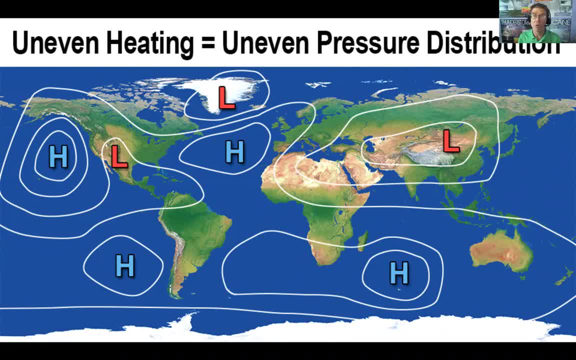 and the Ls stand for low pressure. I'm going to talk a lot more about Hs and Ls and the high pressure and low pressure in the next section. Just think of it as with the area of high pressure you have a few extra air molecules near the surface of the earth And the areas of low 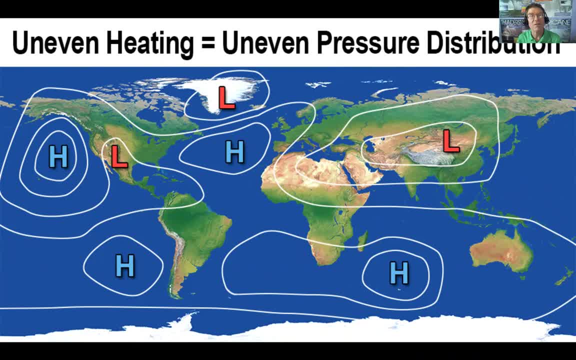 pressure. you have a few less air molecules. You have a few less air molecules near the surface of the earth. These areas of high and low pressure start to form up over the earth. Now if you look at this, you see that the low pressure is forming up over the larger land masses And that goes back. 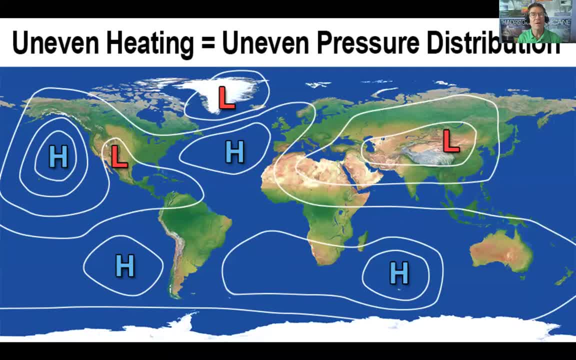 to the reason. The reason that is is because, if we go back to thinking about the land heating up faster than the water, Remember that sunlight passes through the air and then the air strikes the ground and the ground starts to warm up the air from below And that process happens much. 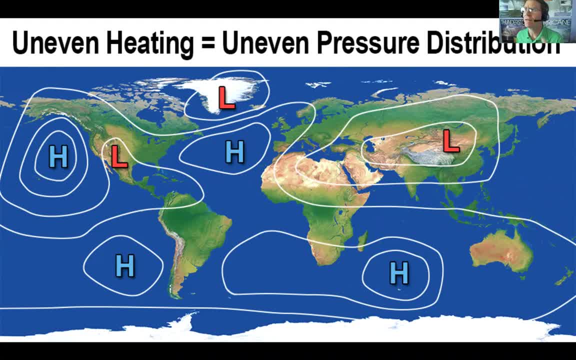 faster over the land, over the water. And this is if you imagine the concept of how about a hot air balloon? You got the pilot and the hot air balloon Pilot turns on the burner. What happens? That balloon starts to float up. Well, as the sunlight starts. 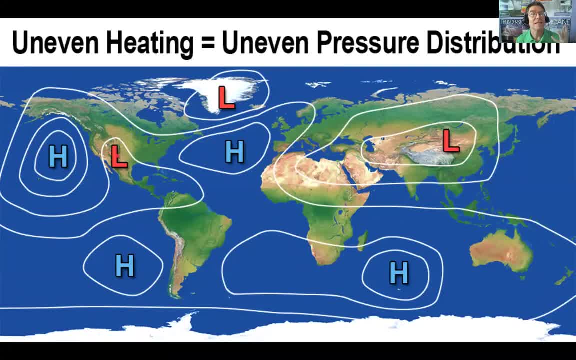 to heat up the air, or I should say, as the sunlight starts to heat up the ground, the ground then starts to heat up the air. And when you start to heat up that air from below, guess what? It starts to rise just like that hot air balloon. So over the land masses you start to have some. 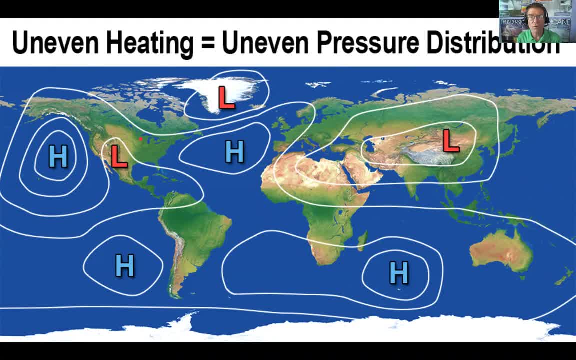 of the air rising up away from the land and that leaves a little void. You have a little less air near the surface, a little less air molecules, versus out over the oceans where it's cooler than the land, because, remember, it takes water a lot longer to heat up. 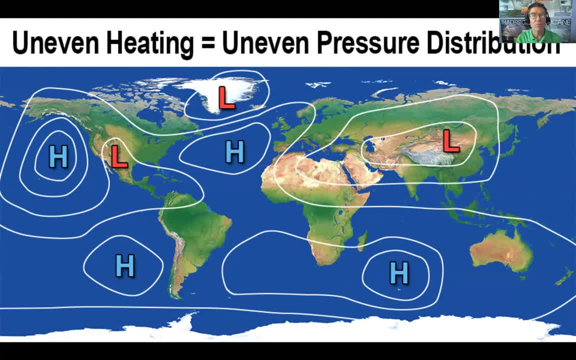 versus the land And so out over the water you kind of, relatively speaking, you have more air molecules near the surface of the water versus over the land, So you end up having this area of high pressure developing. Now I don't want you to think these high pressures and low pressures are 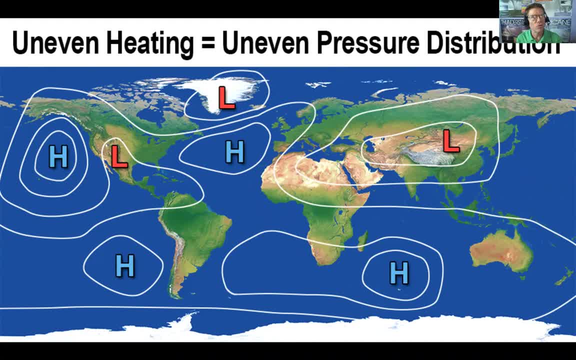 just anchored where they are. As a matter of fact, they actually move along. Did you guys realize that? Well, I'm going to show you a little bit of a picture of what that looks like. So this is a picture of a river of air, And you can see that it's moving. in this river of air, There's always 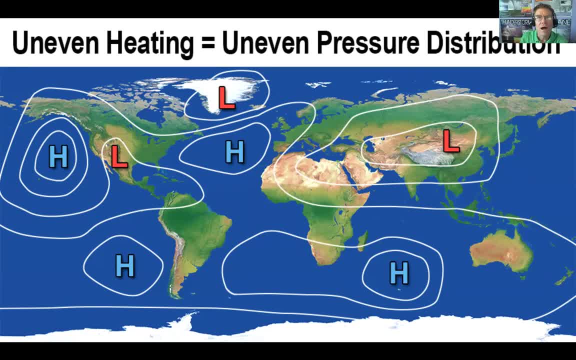 this river of air flowing along. If you've ever gone outside, like say on a summer day, and you've looked at those big white puffy clouds that are floating by, if you look long enough you can actually see they're actually moving. These clouds are actually floating along in this river of air. 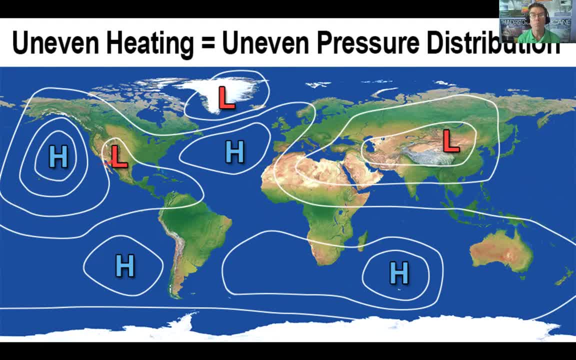 just like a leaf floats along in a creek as it goes down the stream. So these areas of this river of air start moving off. This area of low pressure would move off to the over the desert. It's over the desert southwest kind of right now, where I am. It would drift off over here to the east coast. 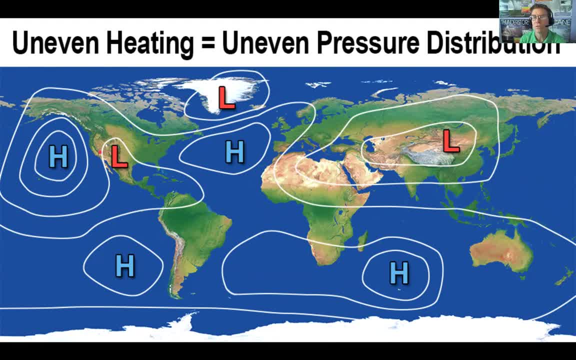 And this area of high pressure over the Pacific Ocean might drift into the west coast. In general, the weather in the United States moves from the west to the east or from the east coast to the west coast. Now I can hear you saying: well, what about hurricanes? They move from. 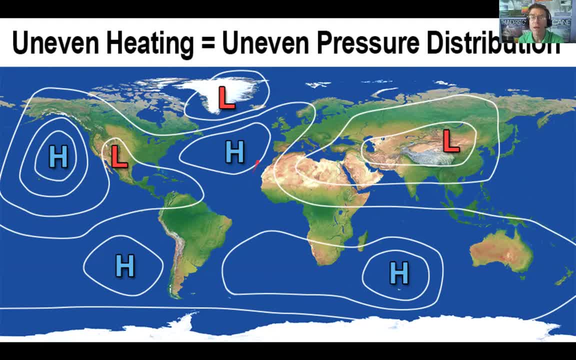 like Africa, up towards us. And that's true. They are a little further south, A little further south of the United States. the winds are actually reversed. They run from the east to the west, But if you watch those hurricanes, they'll travel off the coast of Africa. 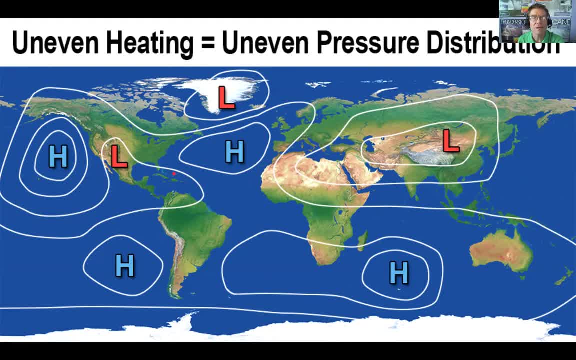 They'll make their way over towards the Bahamas, the Antilles Islands, you know, Cuba and Puerto Rico, And then, as they start to move up here or they start to move off the east coast, you'll see them. They start to make a turn And they'll turn and they'll make this big right-hand. 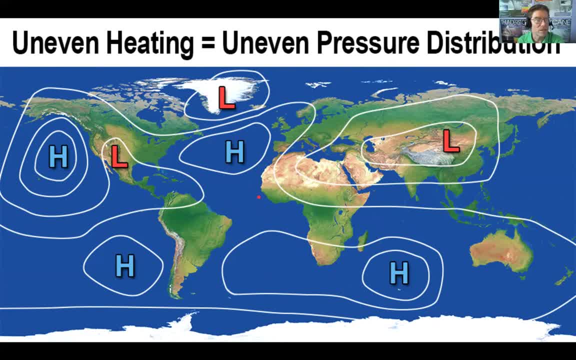 turn. They'll be going north and then they head back in this direction. So they're transitioning from the winds moving from the east to the west up to more where we are in our part of the United States, where the winds move from the west to the east, And you'll see, 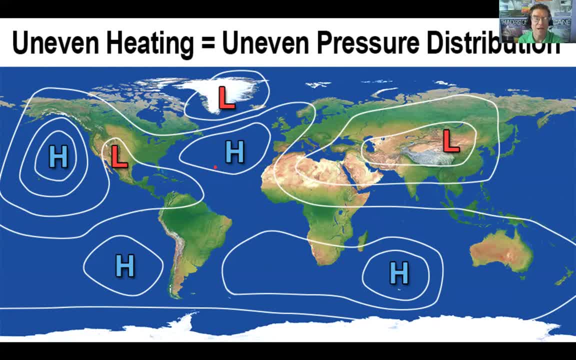 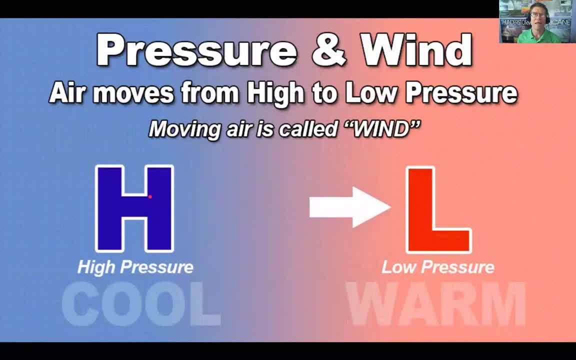 that so that recurve on those hurricanes. it's always kind of interesting to watch. Now, with these areas of high and low pressure, one of the things to keep in mind is that we're all the Earth is always trying to equalize the air pressure. It's always trying to make sure that. 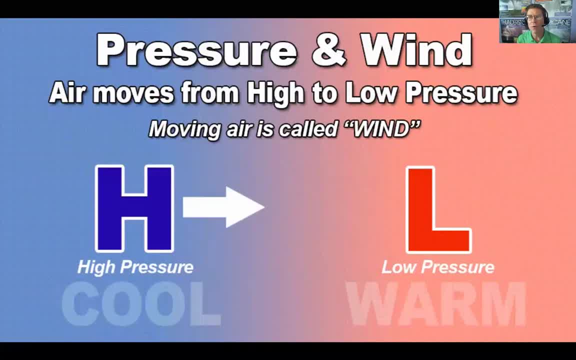 these areas of high and low pressure kind of equalize. It never quite achieves that, But what it does is it takes some of the air molecules in the high pressure, takes it away from the high pressure and moves it towards the low pressure. It's the same concept if you have a bunch of Legos. 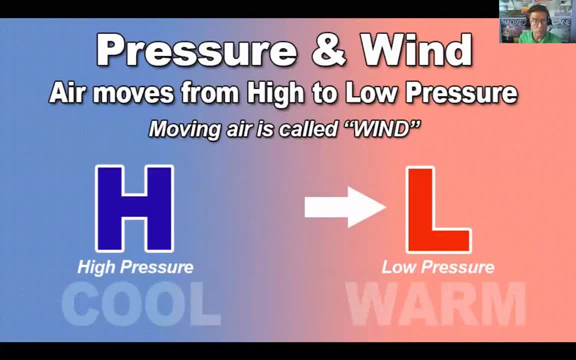 and your friend only has a few Legos. you know you're going to share some of your Legos with your friends, But as we're moving those, the air molecules, from the high pressure and moving them towards the low pressure, as we move those air molecules, that's what gives us our wind. So if 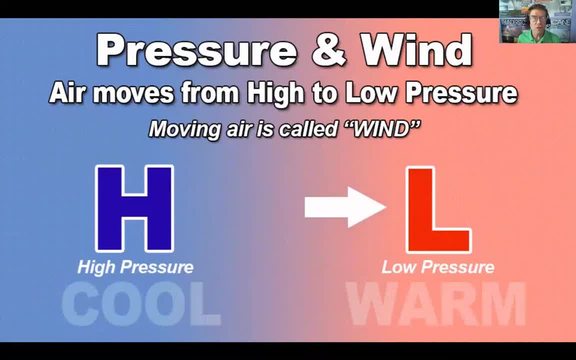 you've ever gone outside on a really windy day. rest assured of you: on one side of you is high pressure, on the other side is an area of low pressure. All right, I got a couple of questions here for you, just to make sure you're paying attention. Let me ask them here to you Because of 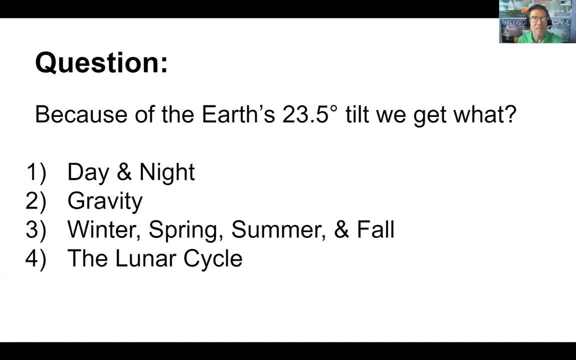 the Earth's tilt on its axis, we get what? Is it one? day and night, Two, gravity, Three, winter, spring, summer or fall, Or four, the lunar cycle. What do you think? Is it one, two, three or? 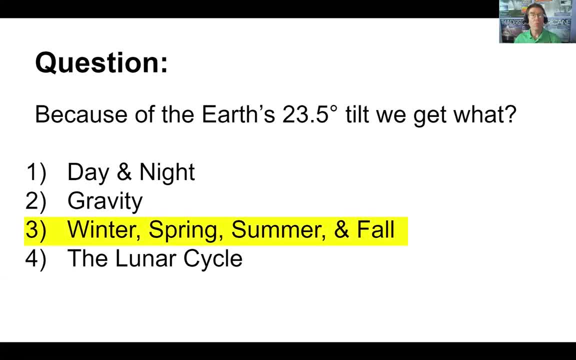 four. Well, if you said three, you nailed it. Remember, because of that Earth's tilt on its axis, we get our winter, spring, summer or fall. We get all of our season, All right. here's question number two. When it's summer in the northern hemisphere. what season is it in the southern hemisphere? Is it one summer, Two winter, Three fall Or four spring? I can hear you already. Y'all are saying, Mr Tim, it's two. When it's summer in the northern hemisphere, it's winter in the southern hemisphere. Good answer. 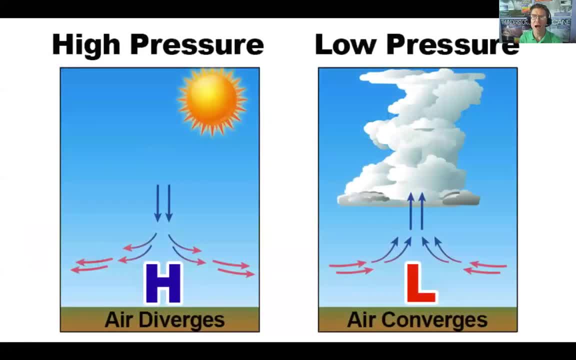 good answer. All right, Let's talk more about these areas of high and low pressure. Like I said, the air is always moving away from high pressure and it's always moving towards low pressure. We're trying to share those air molecules As the air moves away from the high pressure. it kind of creates an empty space above. 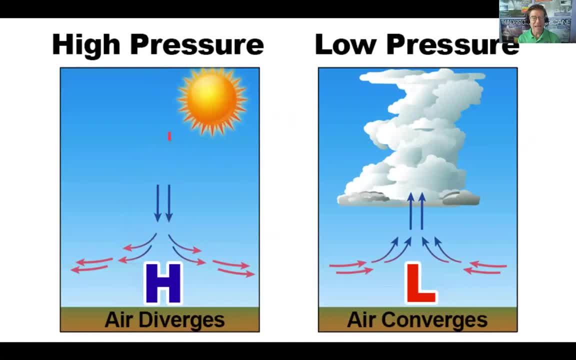 this area of high pressure, So the air above it kind of sinks down Anytime. you have sinking motion in the atmosphere. that's the exact opposite of what you want to get: clouds. So with areas of high pressure you get a lot of sunny skies. That's where we go. 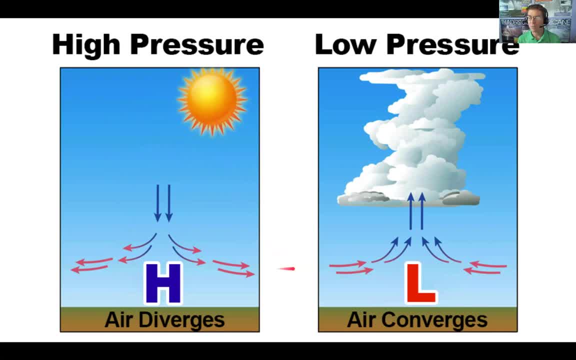 Mr Sun there, But if you look at this, as the air moves in towards the low pressure, it's all getting squeezed together, And when you squeeze it together, it has two choices: It can go down into the ground, or it can go up into the air. It can't go down into the ground, though, because the 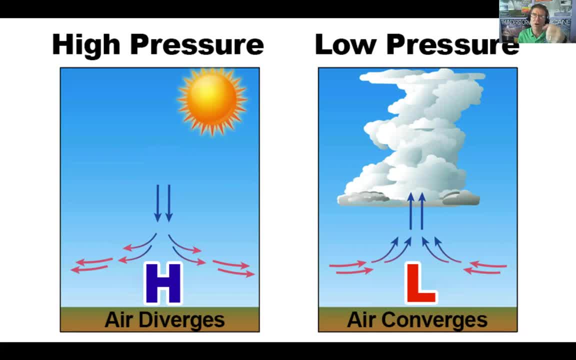 ground is hard So it pops up into the air. It's the same concept. If you hold the toothpaste like this, squeeze it real hard, Don't do this. But if you squeeze it real hard, that toothpaste comes out the opening of the top of the tube. The same thing happens in the atmosphere. 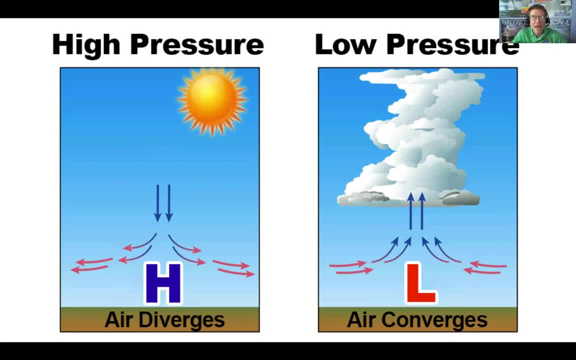 All that air is moving in towards that area of low pressure. It gets squeezed together and it can't go down into the ground, So it goes up into the atmosphere. It goes up into the air And anytime we start getting that lifting motion in the atmosphere, that's exactly what we need to get. 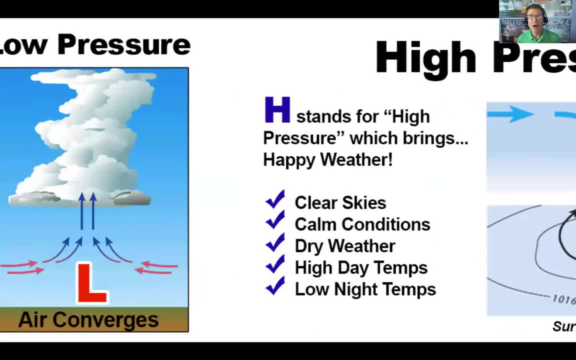 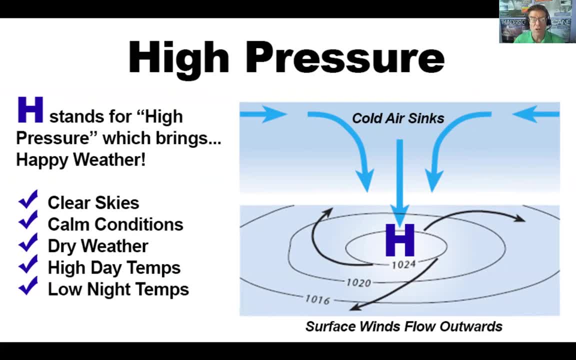 clouds which could eventually lead to thunderstorms. All right, More specific on the high pressure, I tell people to remember the kind of weather you usually get with high pressure: It's the H, is the Q the clue? Because the H stands for high pressure, but it also stands for 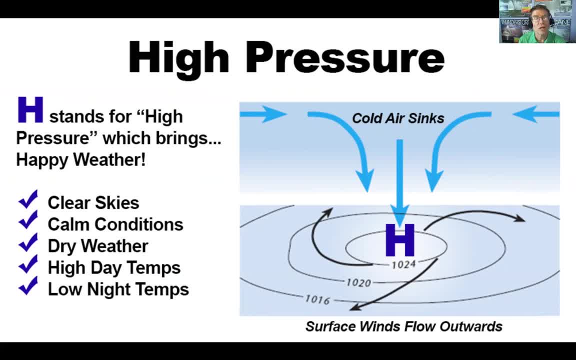 happy weather, Because a lot of times with high pressure you get clear skies, calm conditions, dry weather. It'll be warm during the day because there's lots of sun, And it could actually be a little cool at night. Now this happens more like in the desert part of the United States. But remember how I said. 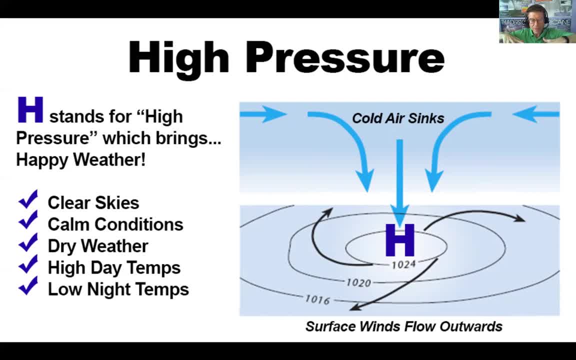 the land cools down quickly. If you have a lot of clouds that actually acts like a blanket, especially at night. It can kind of trap that heat in there. But if you don't have a lot of clouds that land will quickly radiate the heat back out and it starts to cool down. 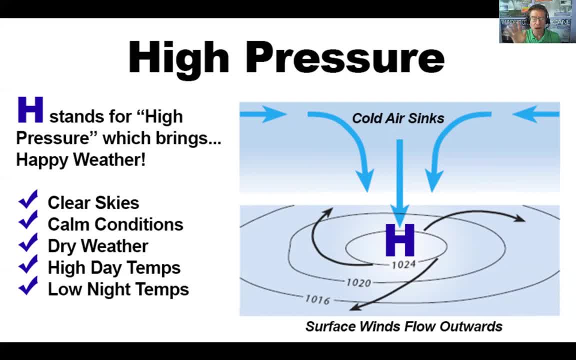 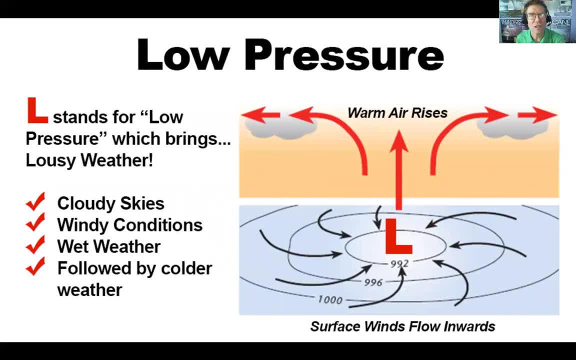 So that's why you can get some cool nights, especially in the desert, on those clear nights when you have that big area of high pressure. The opposite happens with the area of low pressure, And again the L is the clue, Because the L stands for low pressure, but it could also stand for: 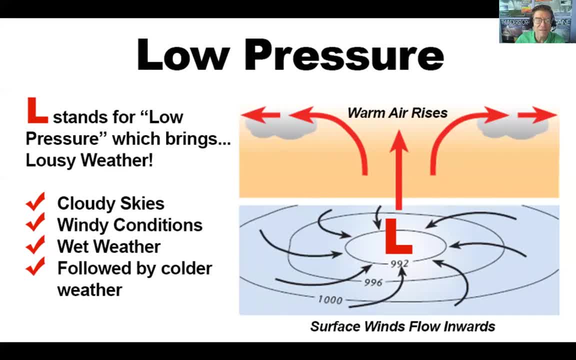 lousy weather, Because so many times with low pressure, we get cloudy skies, windy conditions, wet weather or, if it's cold enough, it could be white weather, And a lot of times it's followed by colder weather, And I'll show you why that is here in just a second. All right, So here's kind. 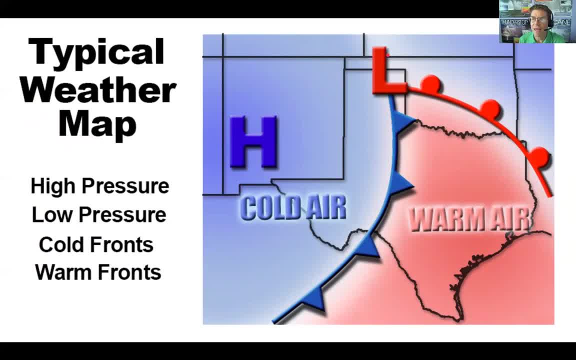 of a typical weather map. We've got the H for the high pressure and we got the L for the low pressure. But now I've added a couple of extra lines on here. I've added a blue line with some blue triangles and a red line with some red semicircles. The red line is a warm front. 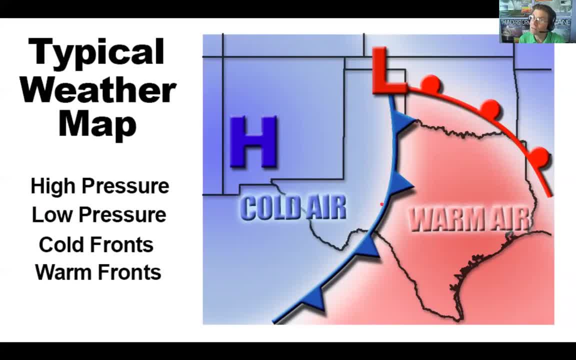 and it's the leading edge of warm air. And the blue line is- you got it- a cold front and it's the leading edge of cold air. You remember how I told you that there's a river of air pushing along the clouds, pushing along the high and low pressure? Well, sometimes that 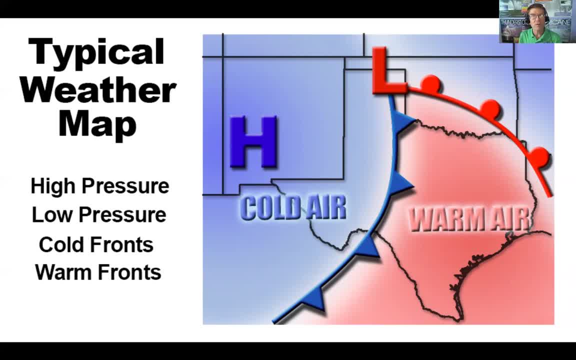 air will push along a chunk of air And sometimes that chunk of air is a cold chunk of air, And sometimes that chunk of air is a warm chunk of air, And these fronts kind of mark the leading edge of which direction those chunks of air are going And you can tell which direction they're. 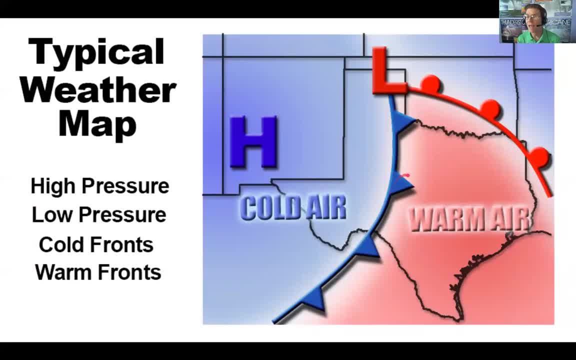 going. With the cold front, the arrows point in the direction that it's going And with the warm front, the semicircles kind of point in the direction they're going. So in this case the cold air is coming out of New Mexico and going into the Texas panhandle area And in this case 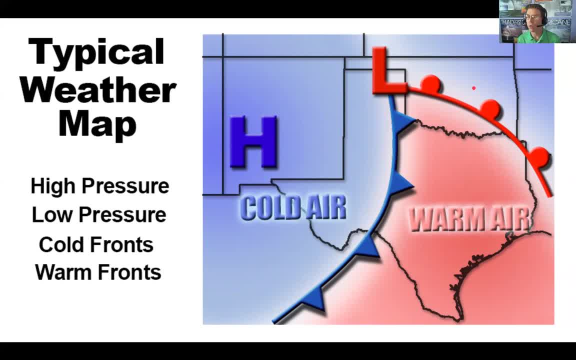 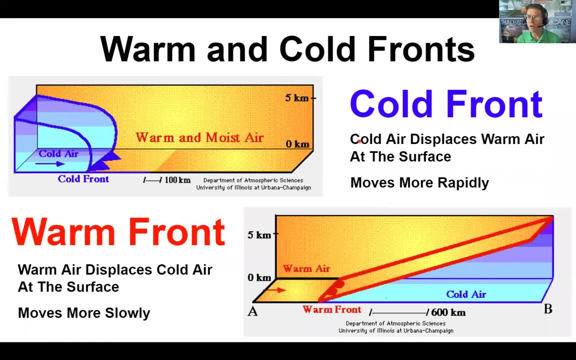 the warm air. the warm air is moving up out of Texas into Oklahoma, So let's talk a little bit more about warm fronts and cold fronts. Cold fronts give us probably the more interesting weather. That cold front is like a big wedge of air And that cold air is dense, So it's always 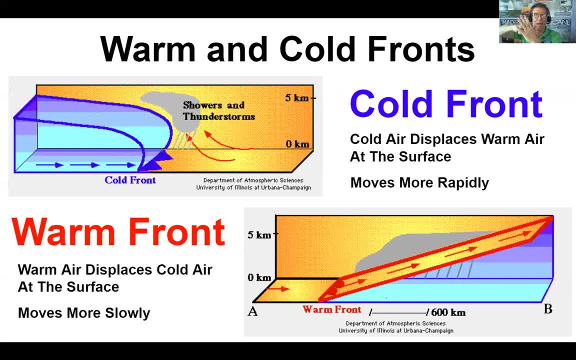 wedging along and it's pushing up the air right along the front edge of that cold front. It's the same concept. if you've ever seen like a bulldozer at, like a construction site, That bulldozer is pushing the dirt, making the puddle, and it's pushing the air And it's pushing the. 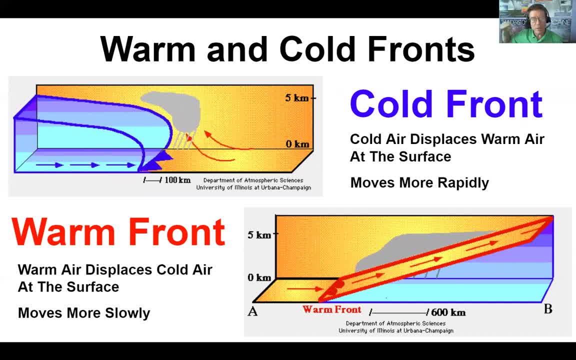 pile bigger, making the pile higher and higher and higher. Well, the same thing as that cold front wedges along through the atmosphere, It's lifting the air right along that cold front, So you can get some thunderstorms and some clouds. You get clouds and thunderstorms if you've got enough. 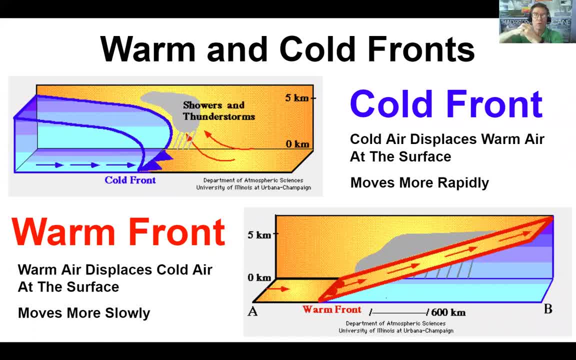 moisture there right along that cold front, So you can get some really intense weather right along that cold front because it's really pushing through and it's really lifting the atmosphere Versus the warm front which is the graphic down here on the bottom. Yes, there is some lifting. 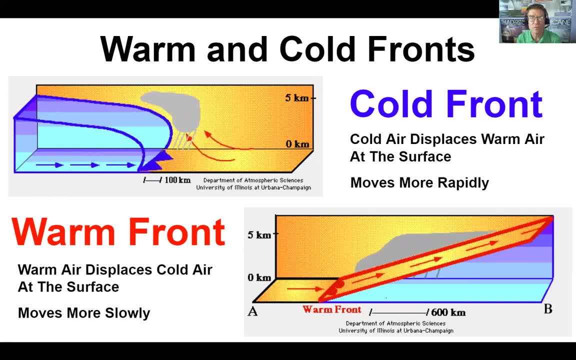 but it's not very steep and it's not very fast. The warm fronts move slower than the cold fronts. It's the same idea if you've ever, like, had a- oh you know- a shopping cart, If you've ever taken a shopping cart at a grocery store and you push it into the grocery store many times. 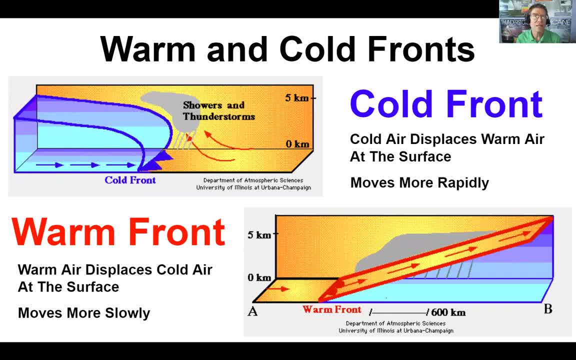 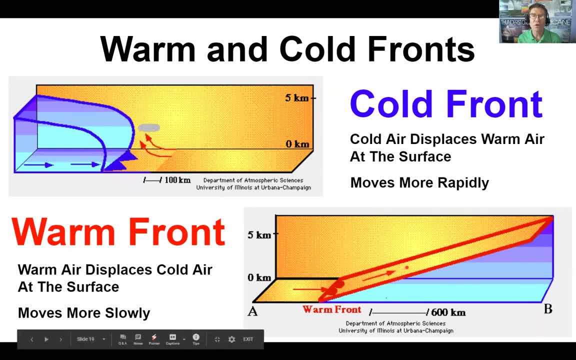 you kind of go up like a little ramp to get into the grocery store. Yes, you did go up, but it wasn't very steep and it wasn't very hard. Same thing with the warm front. Yes, the warm air does kind of slide up over the cooler air it's replacing And you do get maybe some clouds. 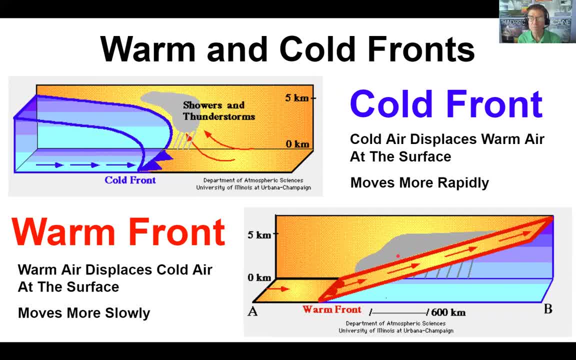 maybe some light rain drizzle, maybe some snow flurries, But it's nothing like the kind of lift that we get right along that cold front as it wedges right along through the atmosphere So we can get our most vigorous and interesting weather right along that cold front. All right, 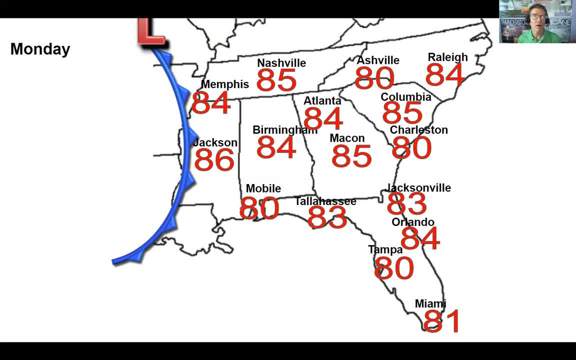 I've got a demonstration of what a cold front moving through part of the southeast part of the US. It's pretty much the same no matter where you are in the United States, So you can just imagine the same things where you are in the United States. But in this case, this is the 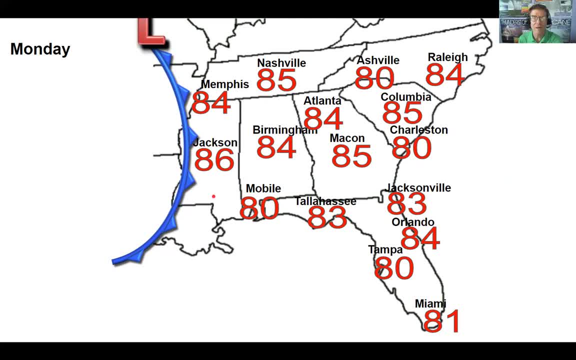 southeast part of the United States And I just made up this. temperatures made up the weather. So let's pretend it's Monday. You got a cold front just getting ready to come into the southeast part of the United States. You see, the cold front kind. 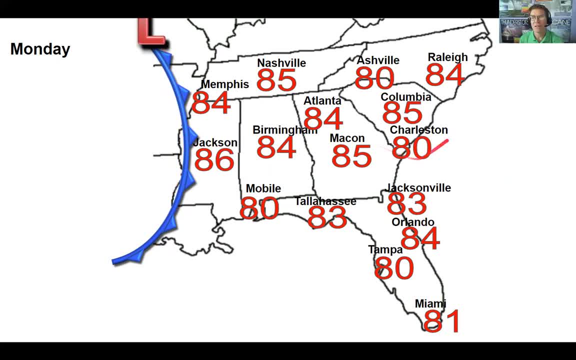 of dangling down from this area of low pressure over Missouri And you can see it's a nice warm, sunny day across the southeast. I shouldn't say sunny, It's just a nice warm day across the southeast where you've got temperatures in the mid 80s in Mississippi, Alabama, Atlanta, Right. 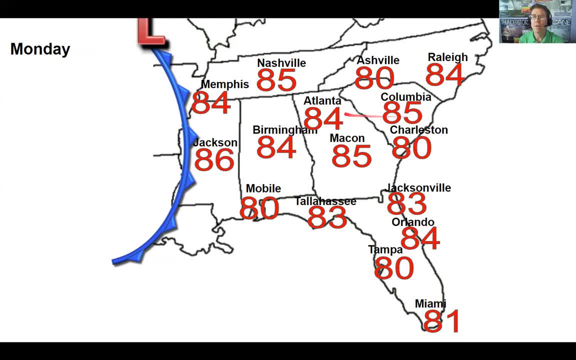 along the coast. maybe a little cooler near the ocean, But really a nice, nice day, All right. So let me jump forward here 24 hours And we'll see what happens. So now you see, the cold front has moved about halfway across the area. 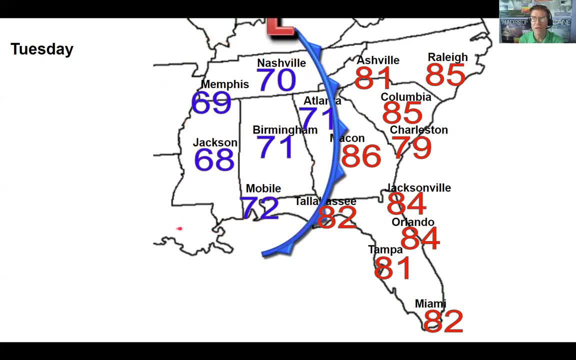 And look at this: On the backside of that cold front is where that cooler air is. So what was in the mid 80s for like Jackson, is now in the upper 60s, But out ahead of the cold front in what we. 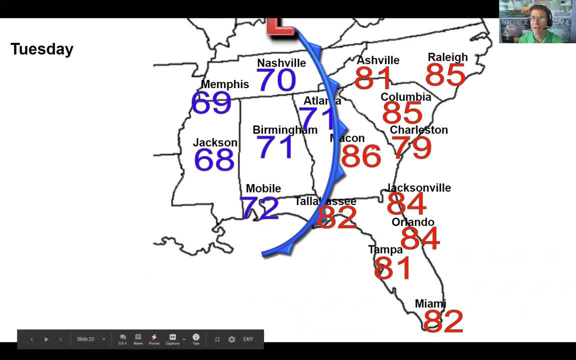 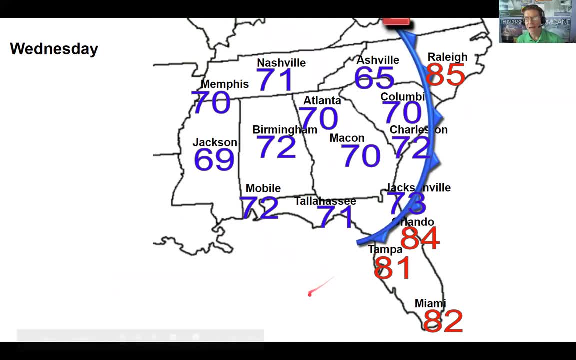 call the warm sector. it's still toasty warm. You can see those mid 80s everywhere except in Charleston. It's just slightly cooler since they're right on the coast there. Now, if we jump ahead another 24 hours now, the cold front has made it a fair way across, actually made it all the way to. 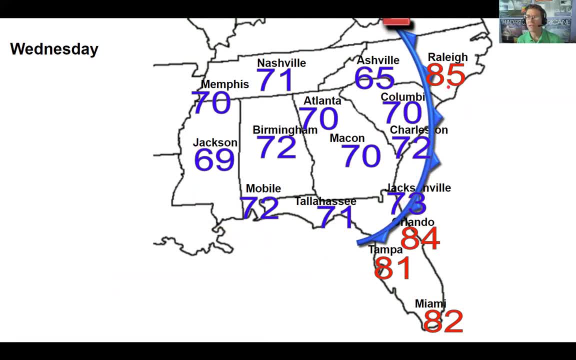 Florida. You've got cold air across the whole area And just still a little. Raleigh is still in the warm sector And it quite didn't make it all the way down into Florida, So they're still warm there in central and southern Florida. All right, So let me jump back 48 hours back to Monday, But instead 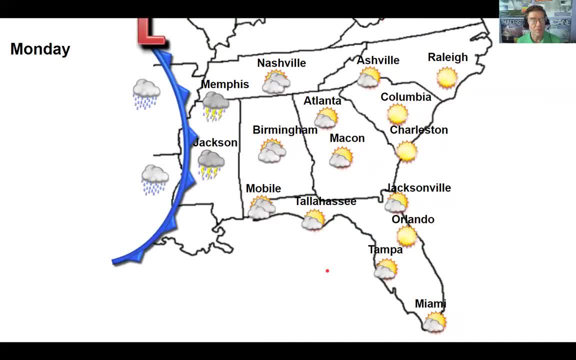 this time of showing you the temperatures, we'll show you the weather associated with that cold front. So again, you can tell which direction that cold front is going by those blue arrows And you can see right along that cold front. you've got the thunderstorms in Memphis and Jackson. 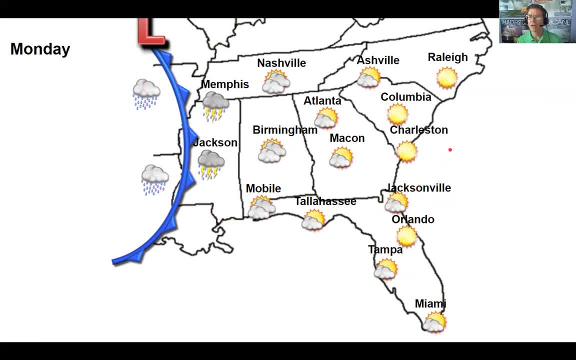 light rain showers trailing behind it. If you look way out of here, ahead of the cold front, Raleigh and Columbia and Charleston, nice sunny skies- They don't even know a cold front's coming. But as you make your way back towards that cold front you can see the clouds increasing And that's that kind. 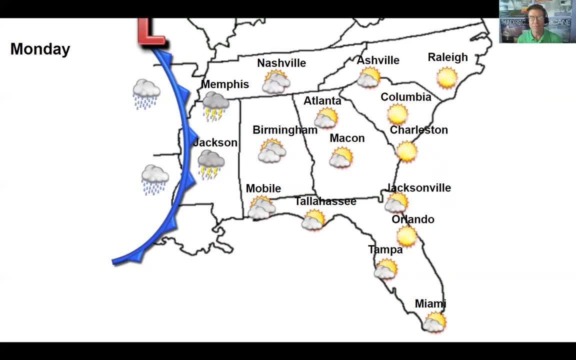 of that lifting motion as that cold front's wedging along. you're getting that lifting motion right along that cold front. Now, if I jump ahead 24 hours now, you can see the thunderstorms are in Asheville, down to Macon, down to Tallahassee. it's starting to cloud up in South Carolina And look at. 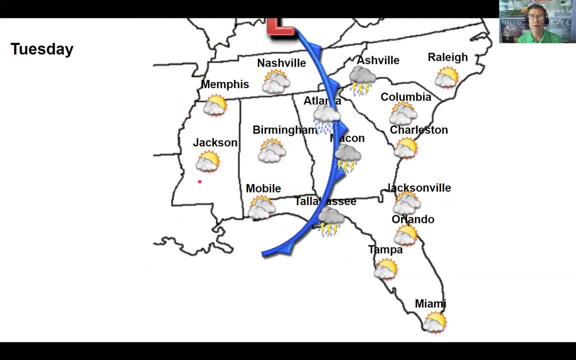 this though: the clouds starting to break up, starting to get some sun way back there in Memphis and Jackson. If I jump ahead again another 24 hours now, you can see the thunderstorms in Raleigh and Orlando. maybe some trailing rain showers there in Charleston. But look at this, it may be cool in. 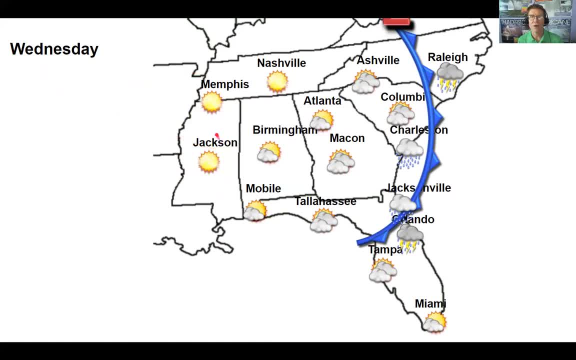 Memphis and Jackson, but that area of high pressure is building in behind that cold front and they have a nice sunny weather there. So that's basically how a cold front will progress across the southeast. It works very similarly in other parts of the country as well. 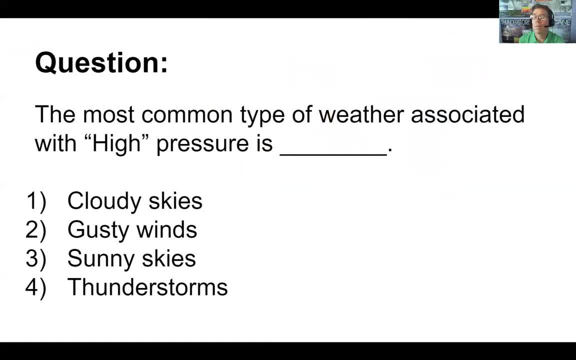 All right, oh yeah, so I got a couple questions for you. The most common type of weather associated with high pressure is what Is it one cloudy skies, two gusty winds, three sunny skies or four thunderstorms? What kind of weather do we get with high pressure? You remember? 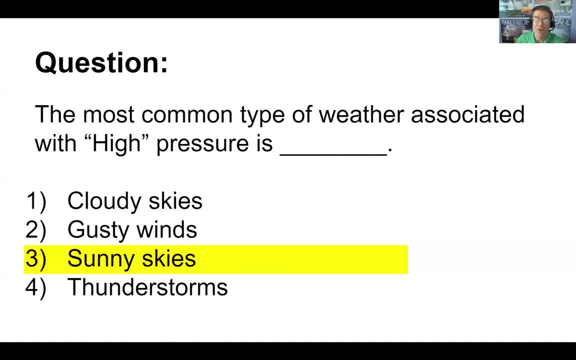 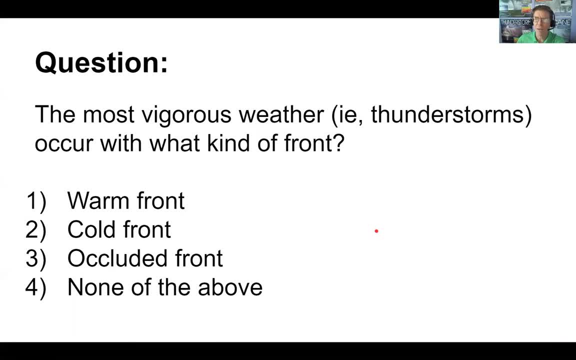 If you remember, with high pressure the H is the key. you get happy weather, And I'll let most people associate happy weather with sunny skies. All right, here's question number two: Most vigorous type of weather, for example thunderstorms, occurs? with what kind of front? 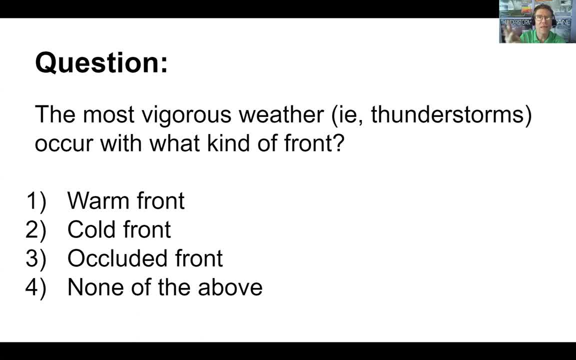 Is it one, the warm front, two, the cold front, three, the occluded front or four, none of the above Occluded front, I didn't even talk about that one. so it's either one or two. So is it the warm front or the cold front that we get thunderstorms? 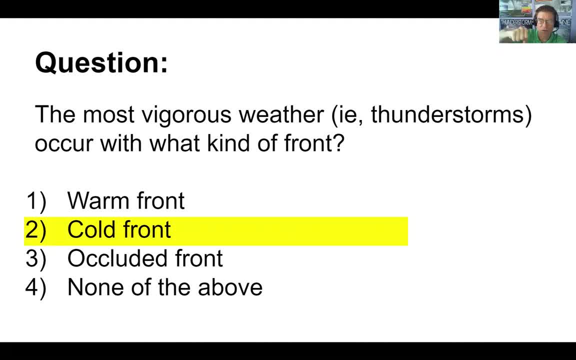 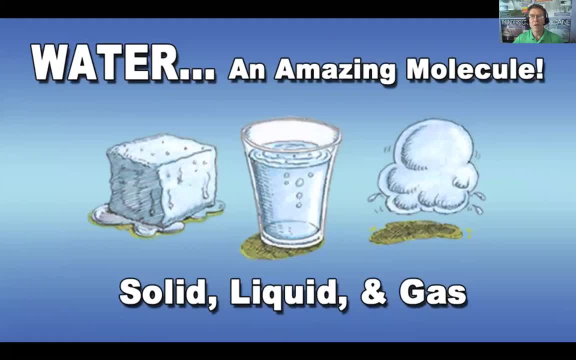 I hope you said cold front number two, because that's where that, as that cold front wedges along, wedges along, it really get that lift right along that cold front. All right, so now we're going to transition and we're going to talk about water as an amazing molecule. 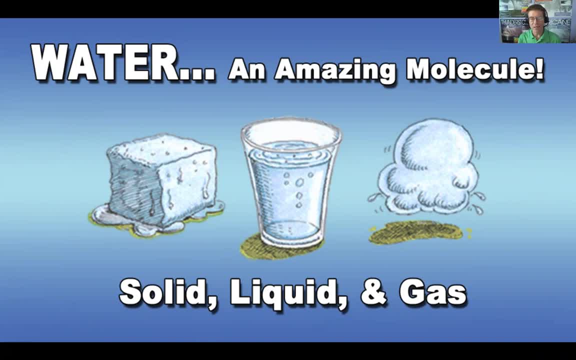 I don't know if you guys have gone over the three states of matter yet- solid, liquid and gas- but you guys, whether you've been formally taught them or not, you probably know what they are because they're all around us. If you're sitting at a desk or a table, that desk or table is a. 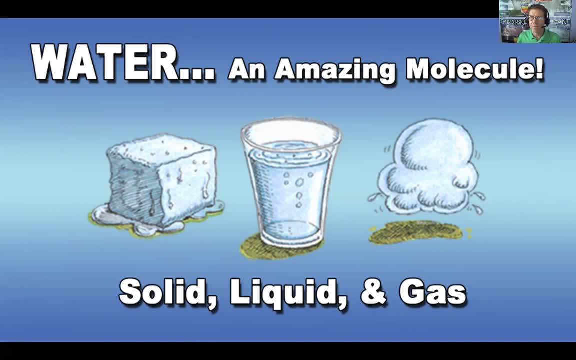 solid, Any water that you drink, any water that you swim in, anything like that. that's a liquid And then a gas is the like, the oxygen and the nitrogen in the air. But water is kind of a neat molecule because it can. 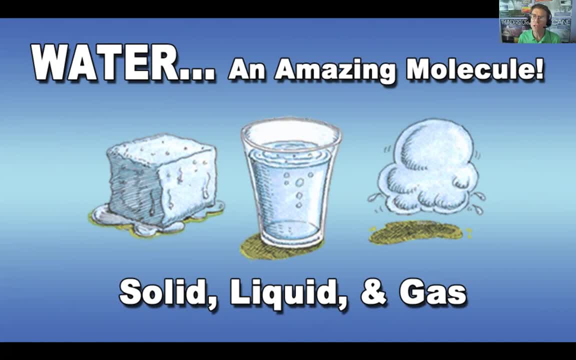 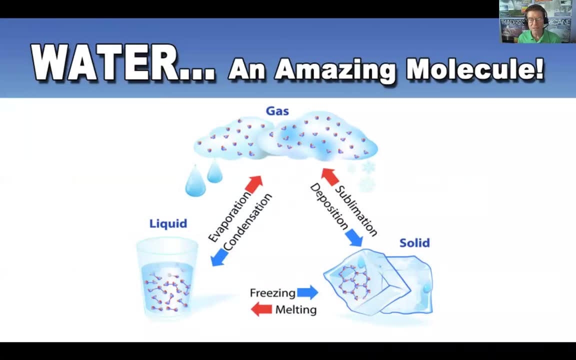 be all three of these states at the same time. in the atmosphere Usually you're one or the other, but water is very unique because it can be all three of these states at the same time. And you guys have all seen this. You're all familiar with liquid water, Of course. 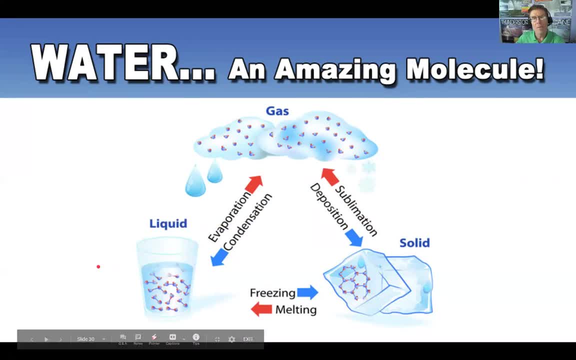 like I mentioned, you drink it, you swim in it, you take a bath and shower in it. But as you add or take away heat from something, you can change its state. So in this case, if you add a bunch of water, you evaporate it and you make it a gas. And that's the same concept when mom or dad put a 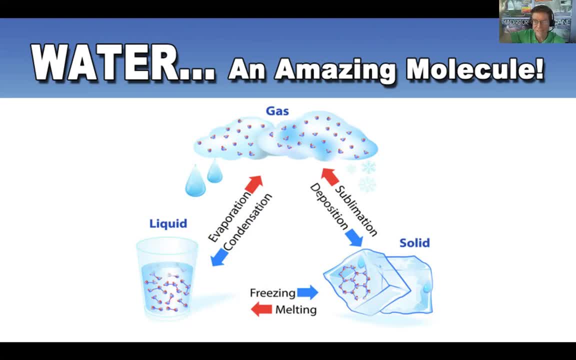 pot of water on the stove and they turn the heat on and it starts to boil. You get that steam coming off of it. That's you changing that liquid water into water vapor, a gas. And the opposite happens If you take water vapor gas and you cool it down. that's called condensation. You'll change that. 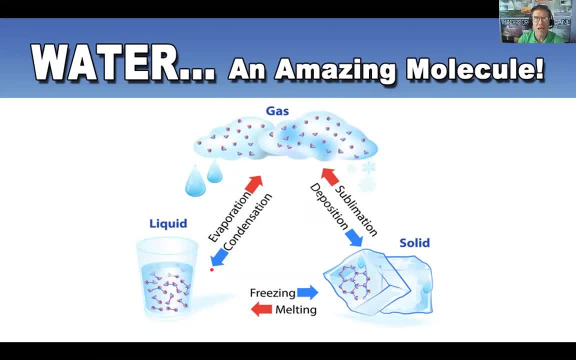 water vapor gas back into a liquid And you've all have seen this on like a hot summer day, if you've got like a soda can or a glass of ice water or a lemonade, All of a sudden on the side of that can or glass, these little beads of water. 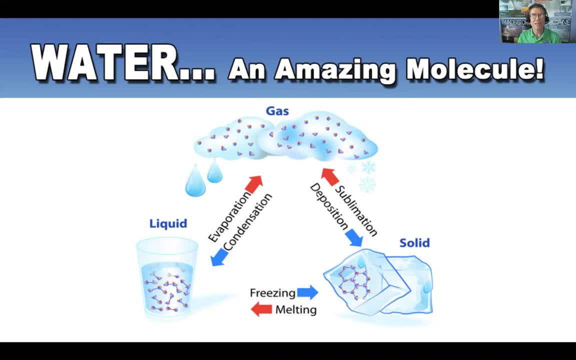 or magic, seemingly magically appear. But what's happening is that that warm, moist air is coming in contact with that cold can or that cold glass And it's cooling the air down to the point where the water vapor gas condenses into a little liquid drop on the side of that glass or can. 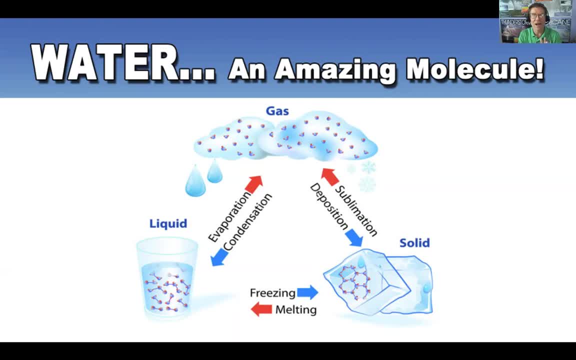 So it's kind of neat. So right there on the side of your can or your glass, you've got that condensation process taking place. You guys are also probably familiar With taking the freezing and melting process. you take liquid water, you put it in the freezer. 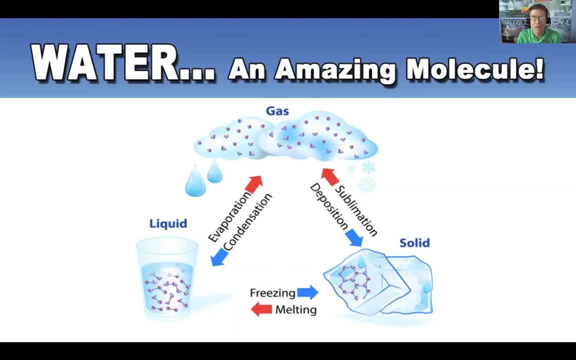 it gets super duper cold in there and it makes solid water ice. That's what ice is. If you take that ice cube out, set it on the counter, it starts to heat that ice cube up and that changes it back from a solid to a liquid As that water melts. that melting process makes that ice cube melt and 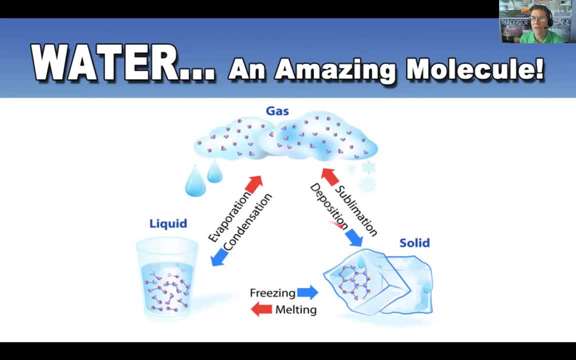 turn back into liquid water. What you may not be as familiar with is going between a solid and a gas, And those words are definitely not familiar with. So what you're going to do is you're going to deposition and sublimation. Don't worry, I'm not going to coerce you on those words, but they're. 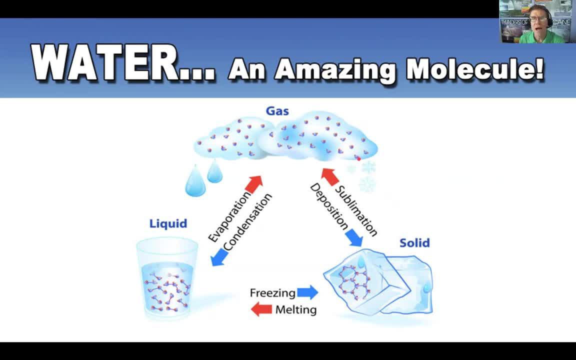 good to know. anyway, You guys may have seen sublimation going from a solid to a gas, maybe around like Halloween time, If someone's ever had like a witch's brew. they take that big chunk of white dry ice and they put it in the pot And all of a sudden out of that pot comes this white vapor. 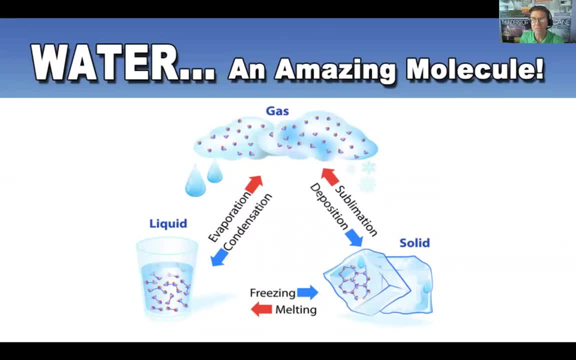 and it kind of flows up and down the sides of the pot. That's that solid, dry ice. It's actually going straight from a solid to a gas And going from a gas and going from a solid to a gas. that's sublimation. But the opposite happens. 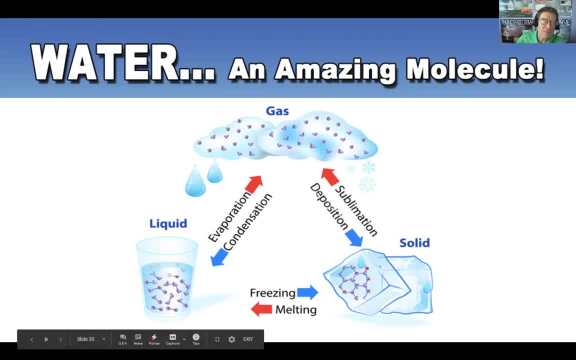 when you go from a gas to a solid and that's called deposition. And that happens a lot at the top of your thunderstorms, In your thunderstorms, even on the warmest day of the summer, at the very top of the thunderstorms, it's super duper cold up there. Remember, as you get further away from. 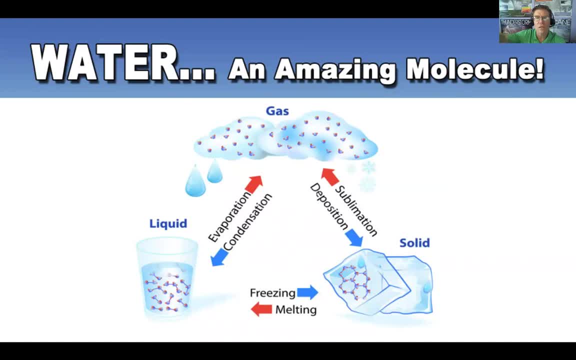 the earth, it gets colder. So in the top of those thunderstorms it's really cold. As a matter of fact, even, like I said, on the hottest day of the summer, all the rain that falls down to the ground actually starts off as ice crystals and snowflakes in the top of that thunderstorm. Just what happens. 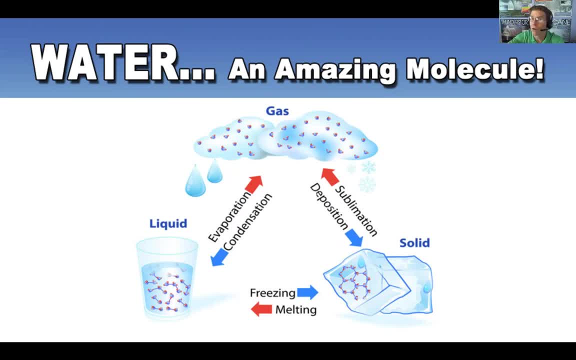 is that the ice crystals and snowflakes float down lower, where it's warmer, And of course you're adding heat to that solid ice and it melts it and it falls as a raindrop. Well, like I said, at the very top of that thunderstorm it's super, duper cold. So any gas, water vapor that's going to. 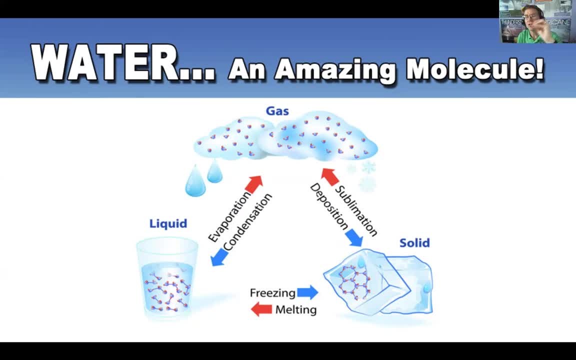 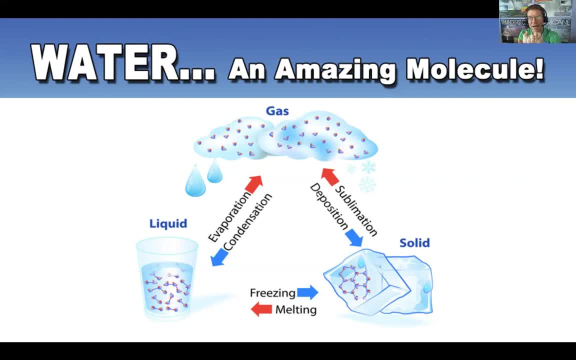 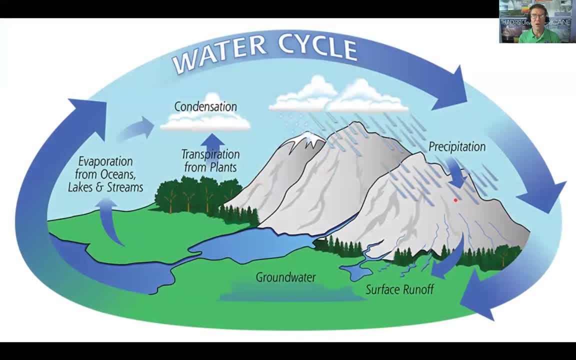 that you guys understand how amazing water is. let's talk about the water cycle Now. you guys all recycle, probably at home or at school, You know. you take a can of soda, you drink it, you throw it in the recycle bin. somebody picks up the bin, they take it to the recycle center. 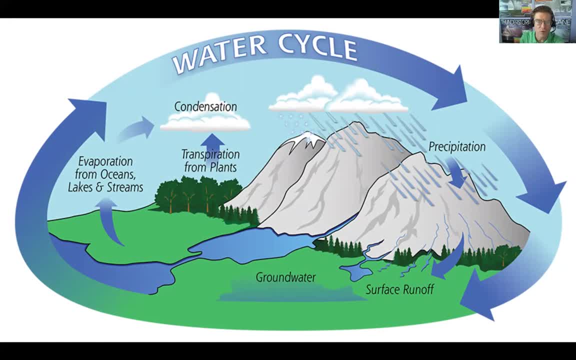 they melt the can down, they pour it into a mold, they make a new can. they put soda in it, give it to you, you drink it, you take the empty can. you throw it in the bin. somebody picks up the. 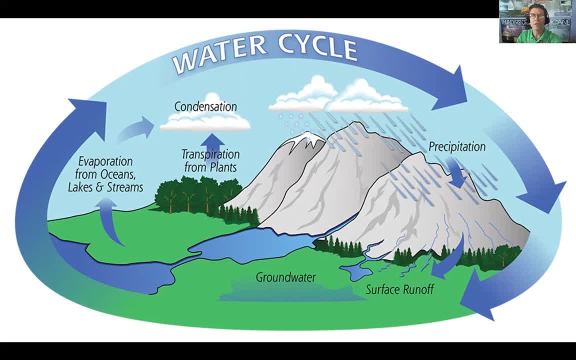 bin. they take it to the recycle center. they melt it down, they pour it into a mold, they make a new can, they put soda in it and you buy it, you drink it, put it in the recycle bin and somebody. 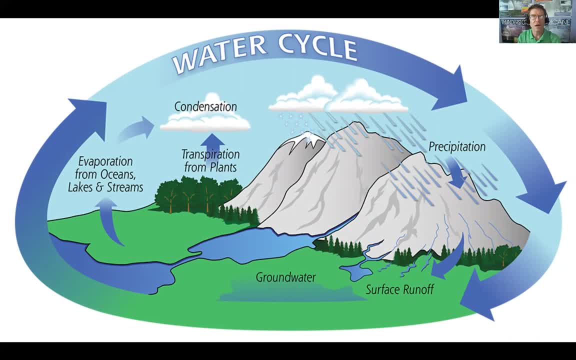 picks it up, and it keeps going like that, on and on and on. So we recycle. we can recycle aluminum cans that way. Well, the same thing happens on the earth, But instead of aluminum cans, we're recycling. we're recycling water, And we can all start with the water. it's called the water cycle. 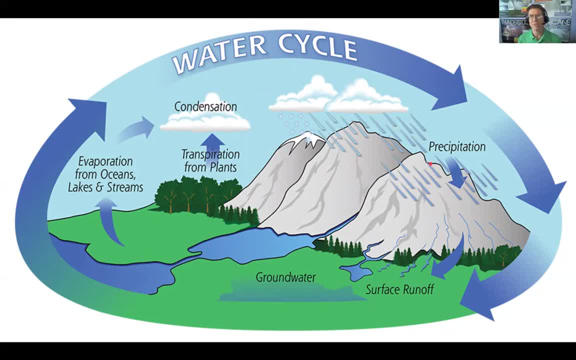 And you know, starts with precipitation. Now, precipitation is just a fancy science word that means either rain or snow. So when you've got precipitation, or rain or snow, you know you get that rain and it runs off, runs off into the lakes and the rivers and eventually into the oceans. 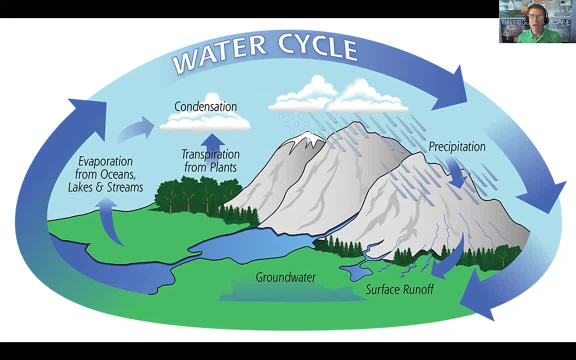 maybe some of that rainwater sinks into the ground, Sunlight shines on the lakes and the rivers and the ocean and evaporates. Remember, it heats up the water a little bit and it evaporates. some of that water changes it from a liquid to a solid and it, I'm sorry. 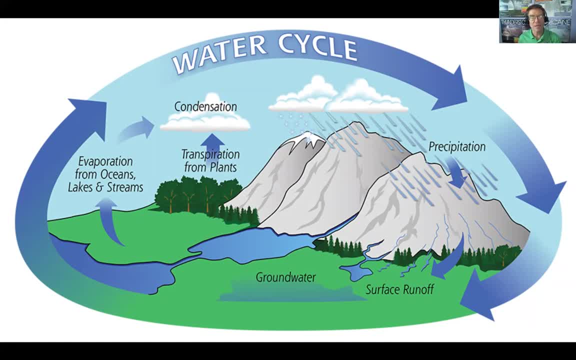 from a liquid to a gas and that gas kind of starts to float up into the air. And that's that evaporation process. As the air, as that water vapor floats higher- remember it gets cooler as you go up higher. the cooling air will then change that water vapor gas back into a liquid, makes a 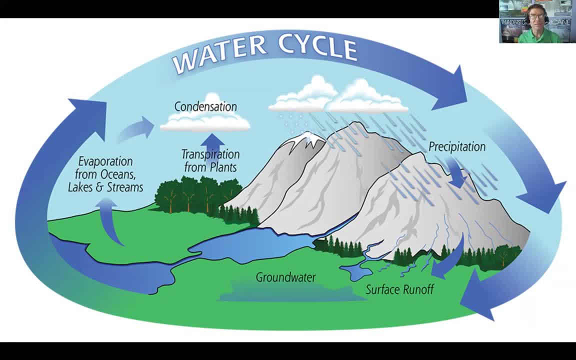 tiny little cloud droplet and that's that condensation process. And as you get more of those cloud droplets joining together, that's eventually you'll get a cloud. And if you get a big enough cloud, guess what? You get either rain or snow at the bottom of it, And then that rain or 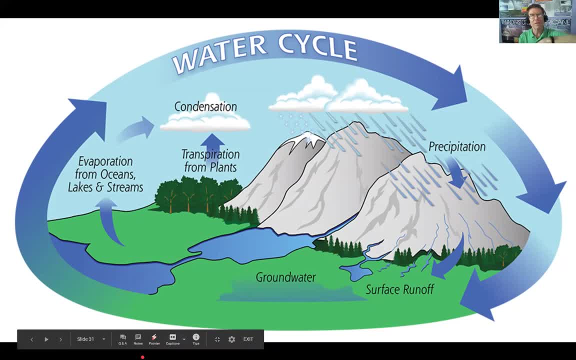 snow. that's the condensation process, And that's the condensation process, And that's the condensation process. And then that rain or snow, you know, the snow falls on the mountain and eventually melts and does the same thing the rainwater does, because that rainwater will run off into the lakes. 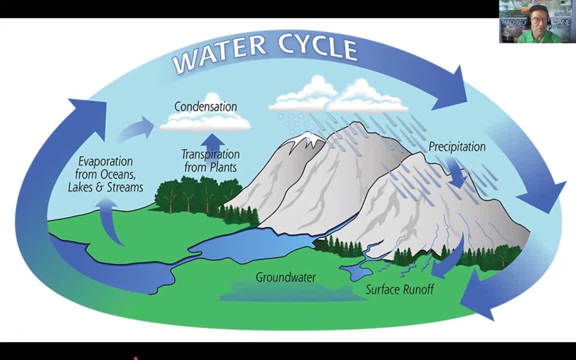 and the rivers and the oceans. The sun shines on the lakes and the rivers and oceans evaporates some of the water. It goes up, It condenses back into tiny little cloud droplets. They get together, they make a bigger cloud and guess what? It rains and snows and the rain runs off into the lakes. 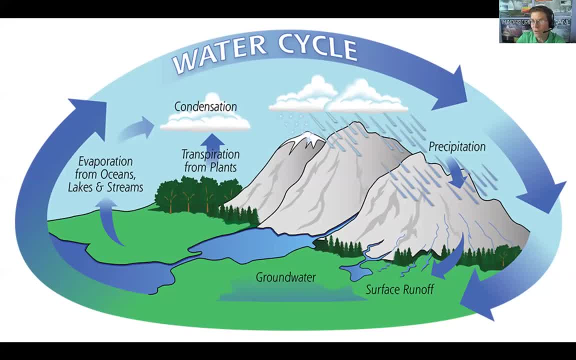 and oceans, and that process just keeps going on and on. Believe it or not, for the last couple thousand years we've neither created nor destroyed water on the earth. It's just going through this water cycle, All right. so now that you guys kind of understand how the water 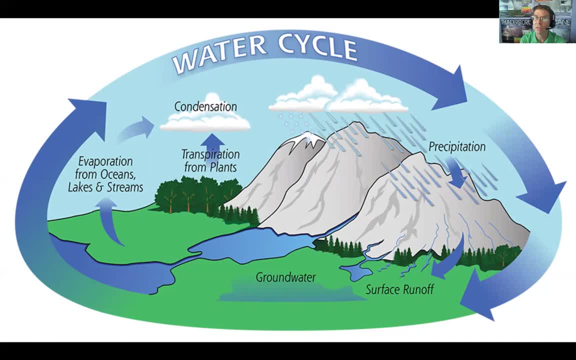 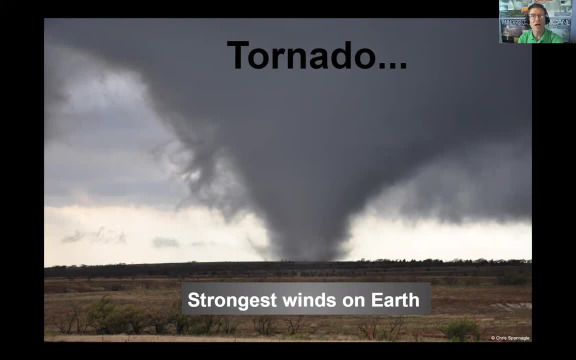 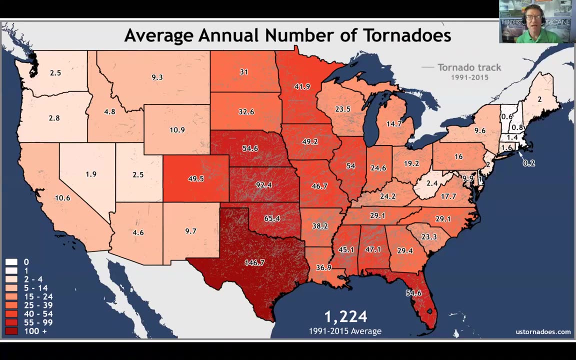 cycle works. I want to get into something a little more interesting. Let's talk about tornadoes. Tornadoes are the strongest winds on the earth. Now, tornadoes occur in every state of the United States, but you can see where the darker red color is here in the middle part of the country. 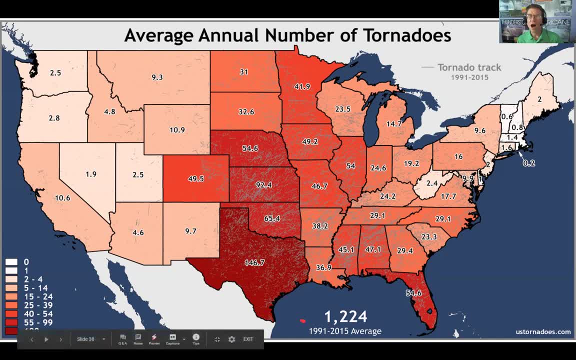 They most often occur in the middle part of the country. Look at this: On average, there's over 1,000 tornadoes in the United States each year and the numbers in each state represent the number on average of tornadoes each year. So you can see Texas, they're in kind. 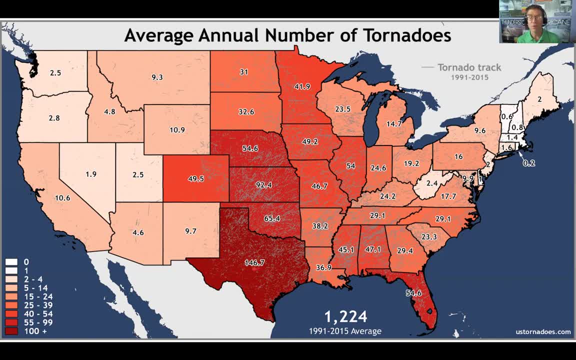 of tornado alley and it's a big state, so they get almost 147, 146 tornadoes a year versus, let's say, a smaller state like Ohio. They only get about 19 tornadoes. but look at this West of the. 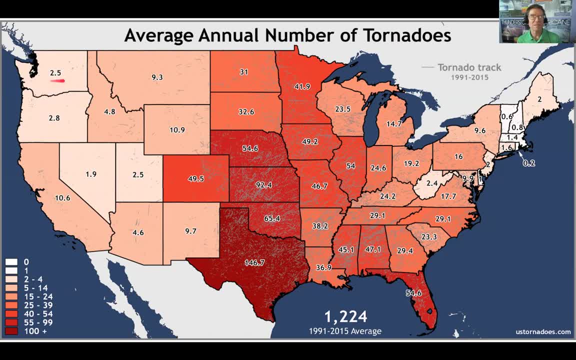 Rocky Mountains. they get less and less tornadoes. Washington State only averages maybe two or three tornadoes a year. California only 10 or 11. But by far the majority of tornadoes occur in the middle part of the country, where we call tornado. 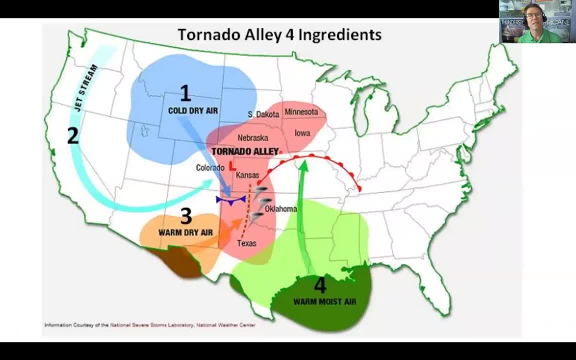 alley, And that tornado alley is simply a place in the United States where we tend to get more tornadoes than any other place. Matter of fact, like I mentioned, the United States sees over 1,000 tornadoes each year, and that's by far more than any other country in the world. So we are the 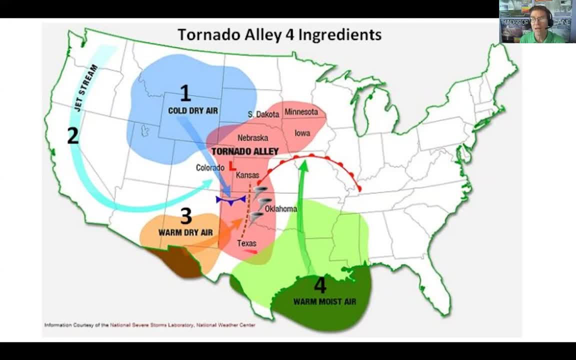 tornado capital of the world. But the middle part of the United States is the tornado capital of the United States and we call that tornado alley. To get a tornado you usually need a thunderstorm And to make a thunderstorm you have to have all the weather ingredients come together, just right. 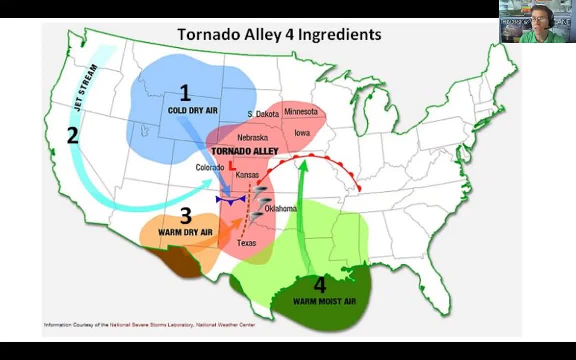 Now, just because you hear thunder, don't think a tornado is coming. Actually, to get a tornado from a thunderstorm is very rare. A whole lot of weather ingredients have to come together just right. So you don't have to be – just because you hear thunder doesn't mean there's a tornado on the way. 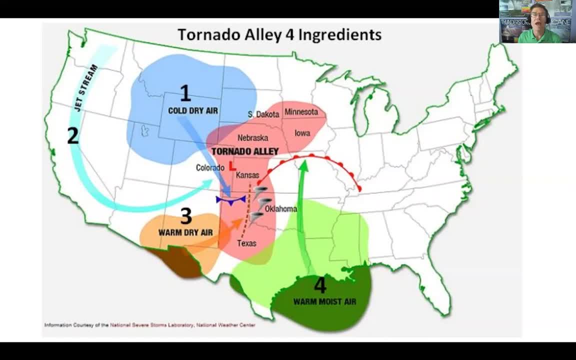 More than likely, it's just going to be a thunderstorm. Every once in a while, when all the weather conditions are just right, you can get that thunderstorm to make that tornado, because all the weather ingredients are just right, And some of those weather ingredients include warm, moist air. 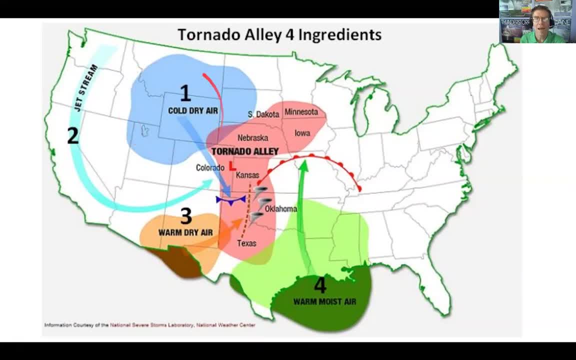 coming out of the Gulf of Mexico, cold, dry air coming out of the northwest part of the United States. you know Montana and Wyoming In the middle part of the atmosphere. you need some warm, dry air coming out of the desert southwest, where I'm located, And you need something called the. 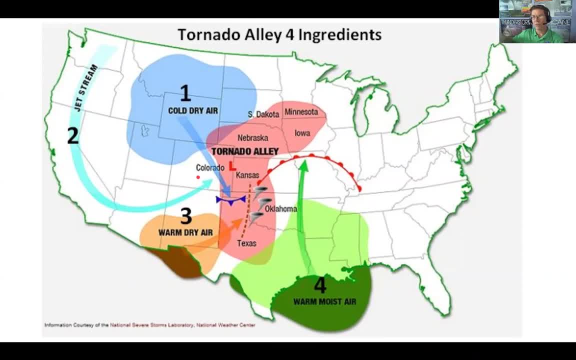 jet stream. You remember how I talked about how the air is always moving along in that big river air. Well, sometimes a little ribbon of that air is actually moving along faster and we call that the jet stream. And this ribbon of air, this jet stream, adds a little extra spin to the atmosphere. 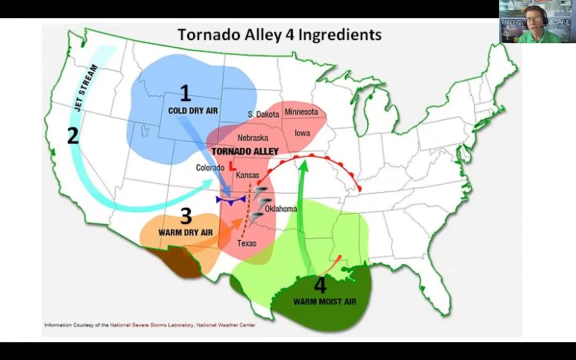 a little extra energy to the atmosphere. And all of these ingredients come together most often in the middle part of the country, and that's why we call it tornado alley. These ingredients can come together in any part of the country, but they most often, like I said, come together most. 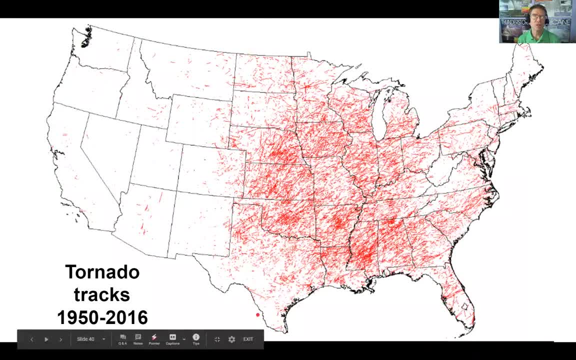 often there in the middle part of the country. All right, I'd like to show this map, because this kind of shows you where the tornadoes occurred. This is the all the tornadoes. each of these little red lines looks like a lot of red spaghetti there. All these red lines indicate: 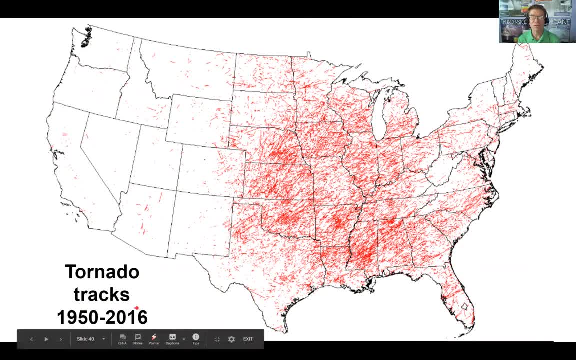 the tornado tracks from 1950 to 2016,. so almost 65 years of tornadoes And you can see. you see a lot. it's hard to see, but there's a lot of just dots where the tornado touched the ground, But you 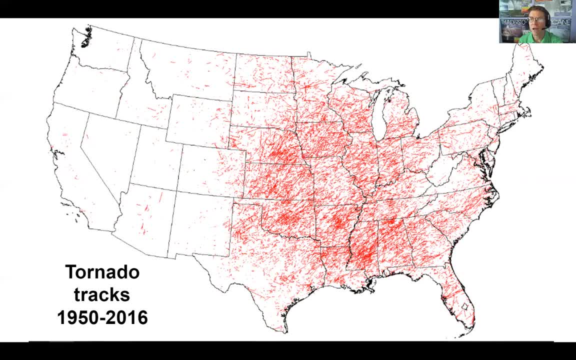 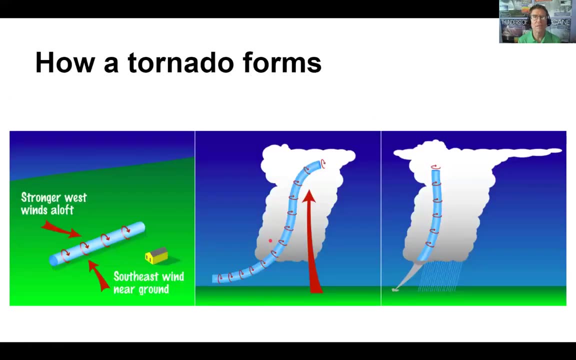 can see some longer lines like up here in Minnesota, in Iowa, but a whole lot of lines. You can kind of see where the tornado alley is here. You can also see down here. there's another kind of maximum of tornadoes down here in Alabama and Mississippi. All right, so how does a tornado form? The 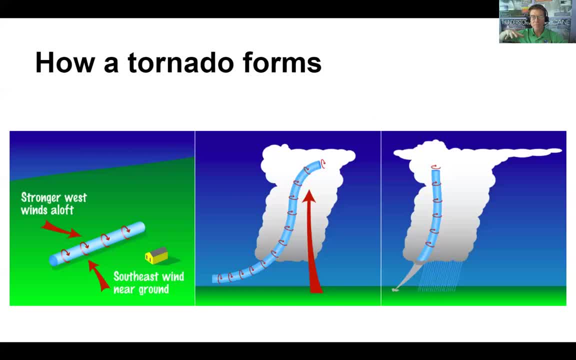 atmosphere is three-dimensional. That means that there's height to it and sometimes what's happening near the ground is different than what's happening up higher in the atmosphere. A lot of times, near the ground you'll get winds from one direction and higher up you'll get winds from another. 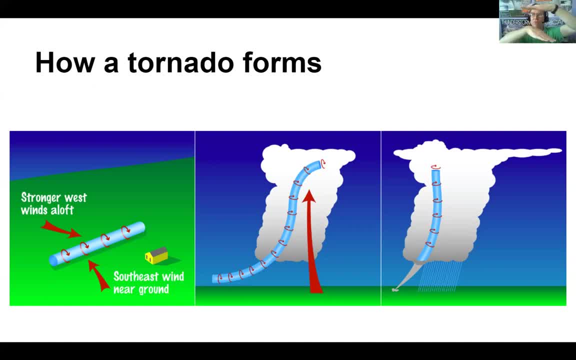 direction. Sometimes they're from the same direction, but sometimes they're from opposite direction. And when they come from opposite directions that kind of gives you a rolling motion. If you've ever helped mom or dad bake like cookie dough or maybe bread dough, you got that. 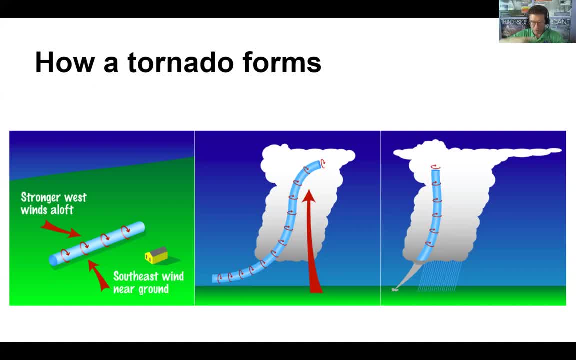 rolling pin and you're rolling it back and forth, back and forth. You've got that rolling motion like this, rolling motion like that. Well, that's what sometimes it's happening with the atmosphere. You've got the winds kind of going opposite each other. It creates that. 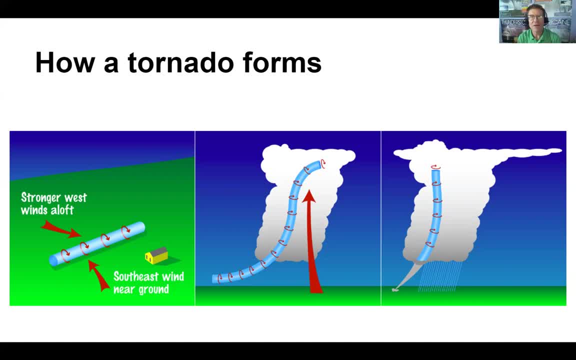 rolling motion. It creates that rolling motion going like this, like this: If conditions are right and you can get a thunderstorm come along, it can take that kind of that horizontal rolling motion and tip it up on its tail, like here in the middle graphic, and now you've got this vertical rotation going. And if the 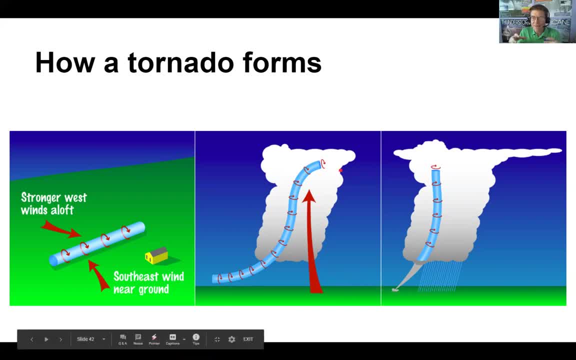 conditions are just right. inside that thunderstorm it'll tighten that circulation down and it'll actually form a little tornado at the bottom of it. The tightening of that circulation is very similar If you've ever watched the Olympics and you've seen the skaters skating around. as she's skating around during her routine. she's. 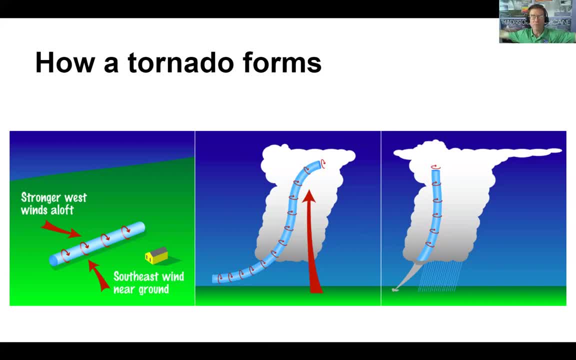 skating, skating. and then, usually at the end of her routine, she'll put out her arms and she'll start to spin around, And then she'll draw her arms into her body and as she draws her arms in, she spins faster and faster and faster. And then, at the very end, she puts out her arms and stops and says: 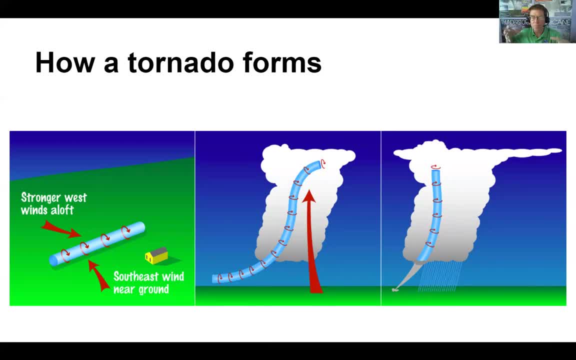 give me a gold medal. Well, something very similar is happening in that thunderstorm. As you tighten that rotation, it gets going faster and faster and faster and eventually, if it gets going fast enough, will spawn that tornado at the bottom of a thunderstorm. All right, so here's some safety. 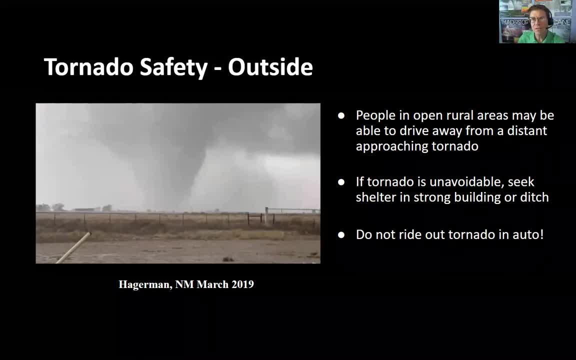 tips for tornadoes. If you're outside and you can see the tornado is far away from you, I tell people you can get in your car and try to drive in the opposite direction of it. But if you are under a tornado warning and you can't see where the tornado is because there's a hill in, 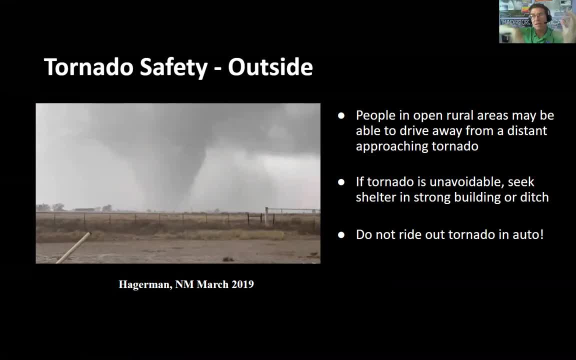 the way. there's trees in the way, buildings in the way, maybe even the clouds are all wrapped around that tornado. do not get into your car. Even the weakest tornadoes can actually toss these cars around. So if you're outside and there's a tornado warning, get inside. If there's no place, 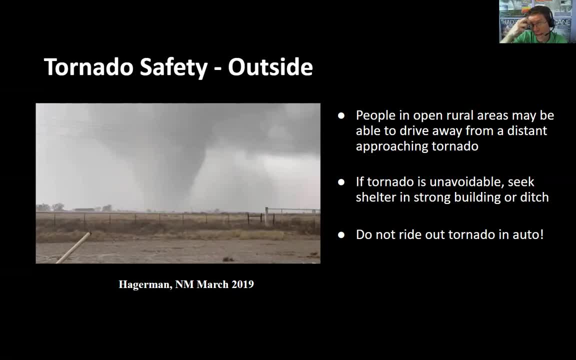 to get to safely. say you're at like one of those soccer complexes with a thousand soccer fields, then you want to find a ditch or a low area to get down into. So if you can't get inside, find that ditch. It's not really the winds of the tornado that hurt people, it's the debris. 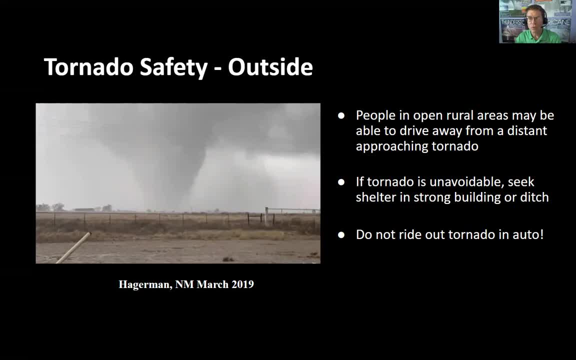 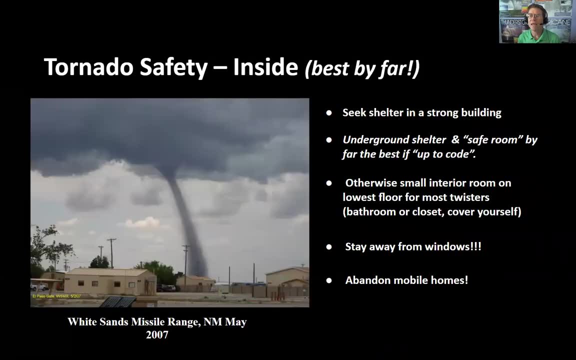 that the tornado picks up and throws around. So you want to get down low, you want to get down kind of in a ditch or something, so all that debris kind of flies over your head. But by far the best place to be is in a building, you know. 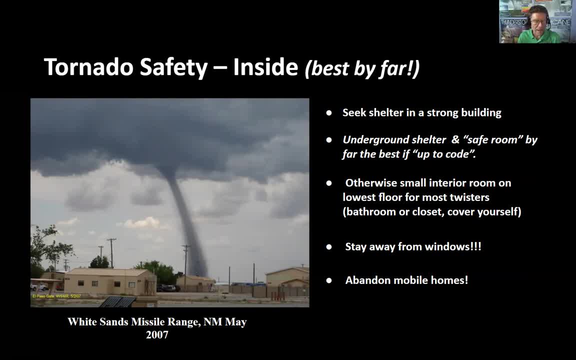 a seek shelter in a strong building like a house, like a school apartment building, a store, something like that. You want to find a safe room. you know, talk to mom or dad. If you're in a place that gets tornadoes. say, mom or dad, where's the safe place to be in our house during a tornado? 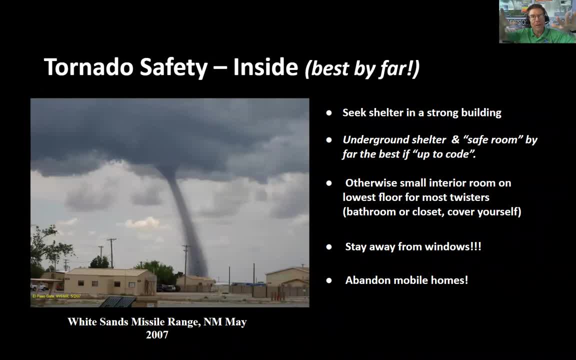 If you have a basement, that's a great place to be. If you don't have a basement, you want to be down on the lowest level of your house, the first floor of your house, the first floor of your apartment building. You want to find a room or a closet right in the 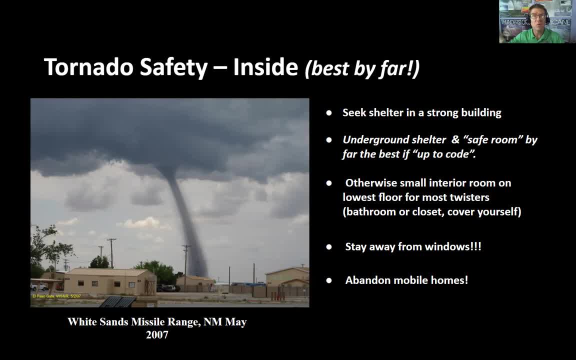 middle of your house or as close to the middle as possible, without any windows, without a skylight. You want as many walls between you and the outside as possible, because all that debris flying around can easily break through windows. If the tornado is strong enough, it can actually push two by. 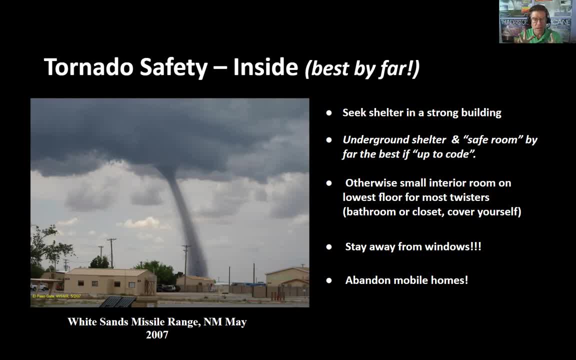 fours through the wall. So if you get a room or a little closet in the middle of your house, you'll be much more safe. You know, I grew up in Oklahoma and whenever there was a tornado warning there, my two brothers and myself, my mom and my dad and our dog would go into this little walking closet. 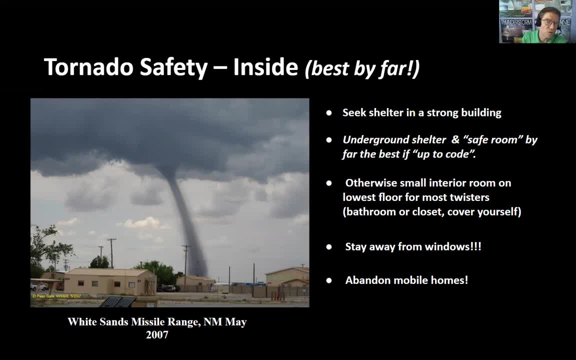 in the middle of our house. We'd have a radio with us and once they said the tornado warning was over, we'd come out Now. thankfully, a tornado never hit our house, but it was just. we knew what to do. You have to have to plan. you have to plan ahead of time. 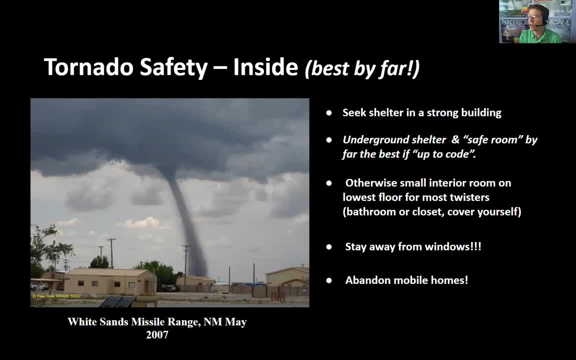 to know what to do, so that when the tornado warning goes off, you're not running around saying, oh, what do we do? What do we do? So always have a plan beforehand to know what to do. Where's your safe room? Where do you go if there's a tornado? Now, if you happen to live in a mobile 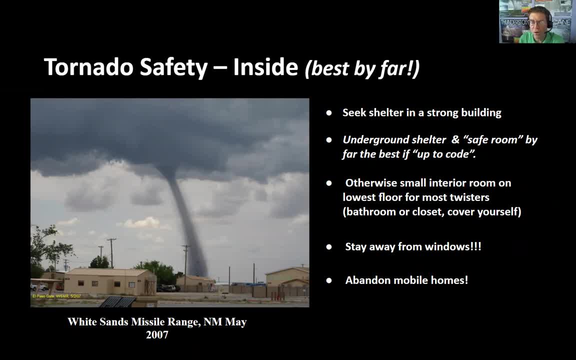 home. mobile homes just aren't safe during a tornado. They're not bolted down to the ground as securely as like a site-built home, so they easily roll over even with the weakest tornado. So but the good news is, a lot of mobile home parks have these community tornado shelters. So 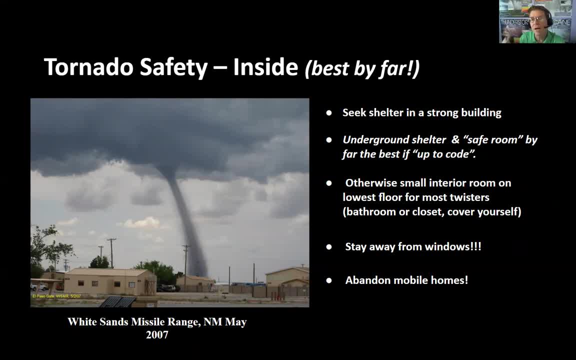 if there's a tornado warning, that's where you go during a tornado. But if you live in a mobile home and don't have a community shelter, ask mom or dad: where's the safe place that I can go real quick during a tornado warning? You know, it might be the store across the street. it might be a. 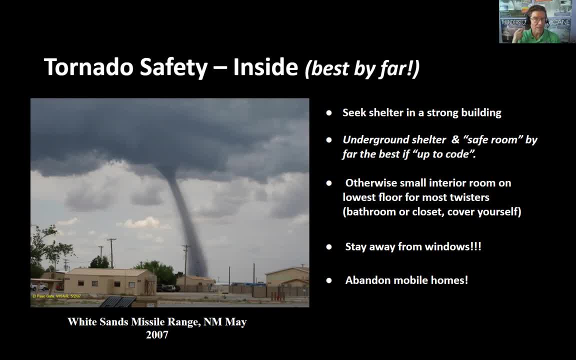 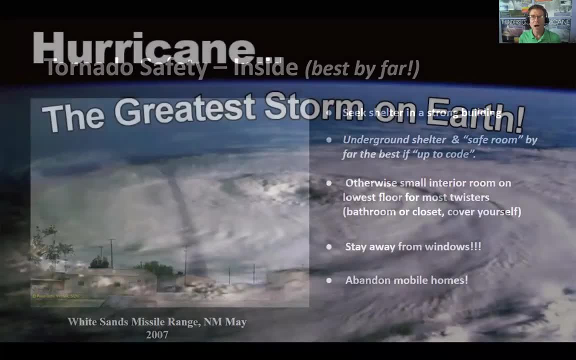 neighbor's house nearby. So again, just make sure that you have a plan in place so that when that tornado warning does come, you are ready for it. But hopefully it never comes, but you need to be ready for it, just in case. All right, we're going to switch gears Now we're going to talk about 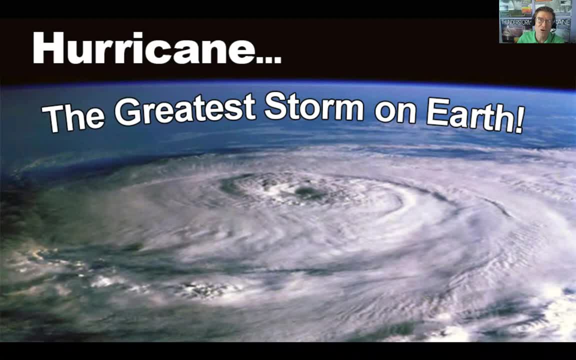 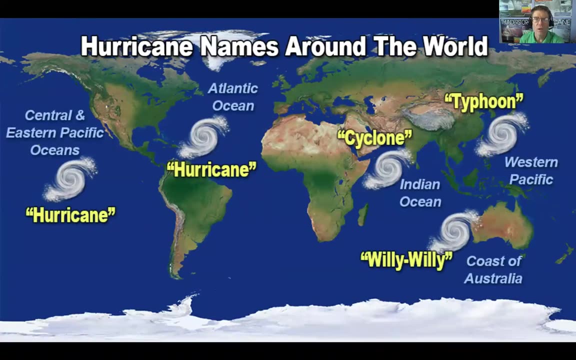 hurricanes. I like to call hurricanes the greatest storm on earth And the reason that the greatest storms are big and these hurricanes. they have so many different weather threats associated with them. Now, hurricanes occur all around the world. You know where we live, in the Atlantic Ocean. 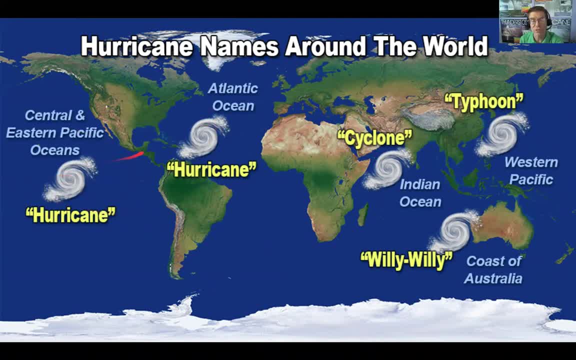 the Gulf of Mexico and the central and eastern part of the Pacific Ocean. of course, they're called hurricanes, That's what we know them as. But look at this Here, towards the western part of the Pacific Ocean, near China, Japan, the Philippines- it's the exact same weather system. 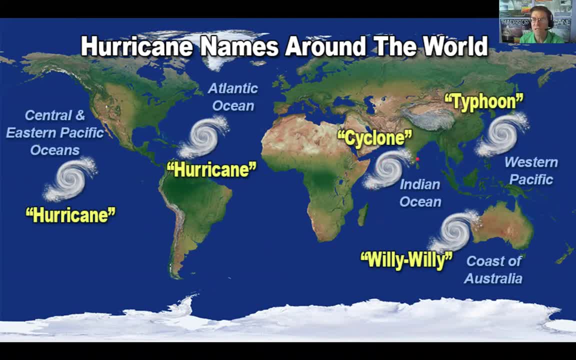 but they're called typhoons. And in the Indian Ocean, near India, Africa, Saudi Arabia, again same weather system as the typhoon and the hurricane, but they're called cyclones. And look at this Off the west coast of Australia: sometimes they're called cyclones and sometimes they're. 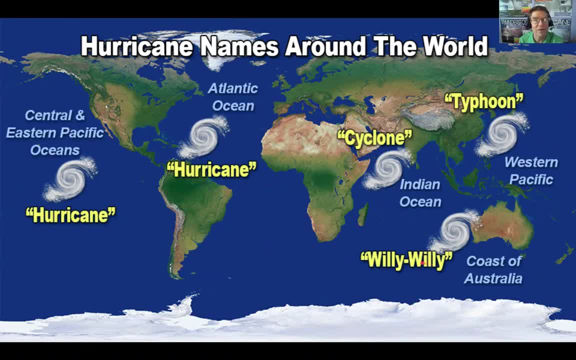 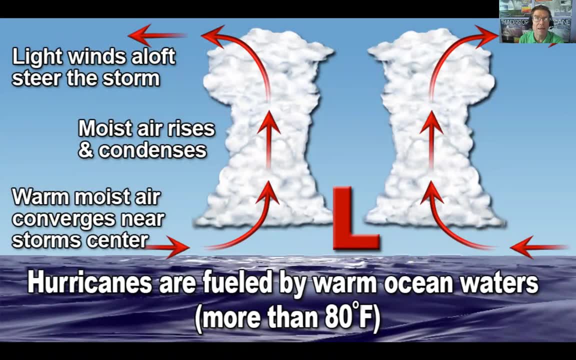 called willy-willies, And that's a very silly name for a very serious storm. let me tell you All right, Inside a hurricane is a big area of low pressure. Remember how I mentioned that low pressure usually brings lousy weather. I can't imagine much more lousy weather than a hurricane. 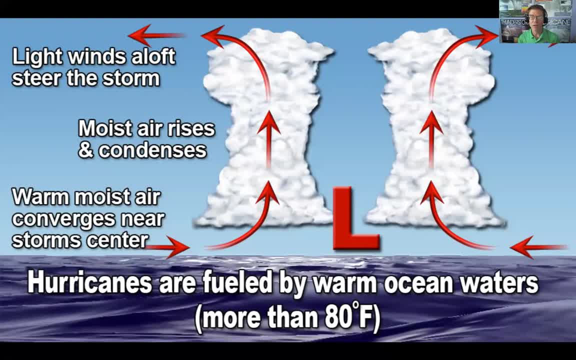 Shouldn't surprise you that at the middle of it is this big area of low pressure. So, this area of low pressure, it takes as fuel to make the hurricane stronger warm ocean waters, And it takes those warm ocean waters and all that warm water vapor air above it and it changes it and 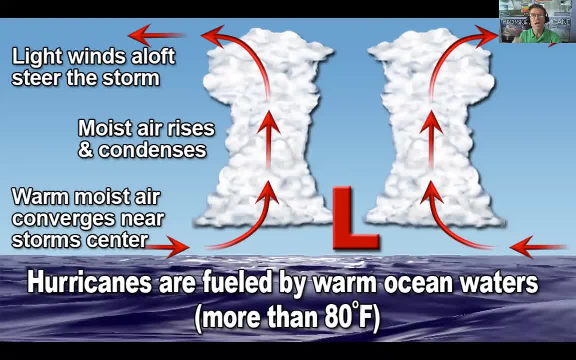 makes it fuel and energy for that hurricane. It's what makes it stronger. Just like you or I get your energy from the food that we eat, the hurricane gets its energy from those warm ocean waters. You know, if you forget to eat breakfast and you don't get a chance to eat breakfast, 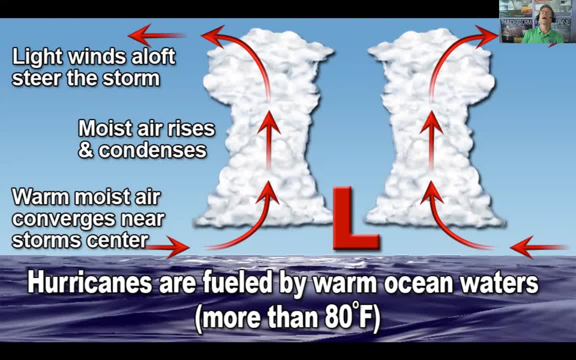 and you don't get a chance to eat lunch. you know, by the afternoon you're going to be laying around going: oh, I'm so tired, Someone please feed me. Well, the same thing happens with the hurricane. If you cut the hurricane off from its fuel source, it immediately starts to weaken You. 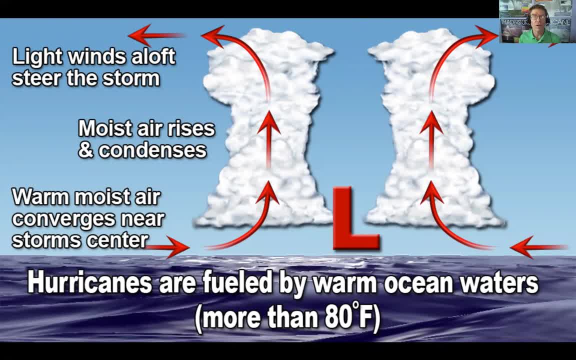 can do that by moving it over colder water or moving it over land, And that's also why we don't get hurricanes, usually during the winter, The waters in the Atlantic Ocean and the Gulf of Mexico are too cool to support a hurricane, But once those waters start to warm up, 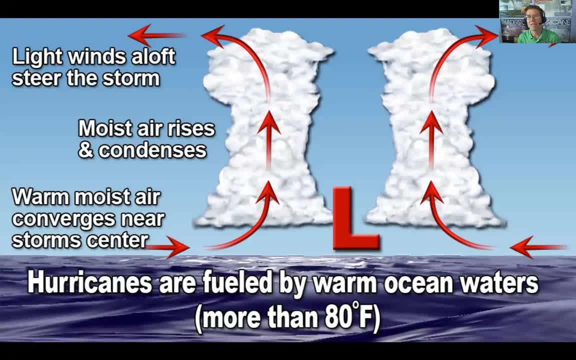 then you can start to form these systems. So that's why you'll see more hurricanes, Because, remember, it takes water longer to warm up. So the water, even in the middle of summer, they're still warming up, But by the time you hit the end of the summer into fall. 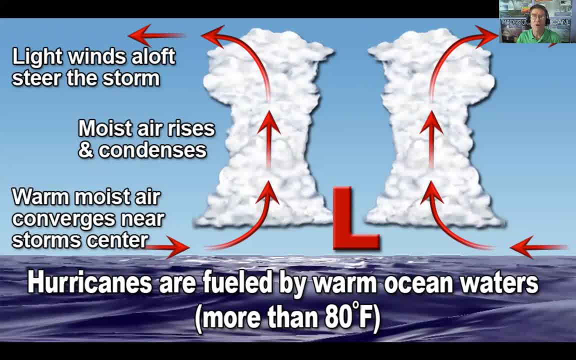 those waters in the Atlantic Ocean and in the Gulf of Mexico are very warm And that's when we get most of our hurricanes in the United States, especially there on the Gulf Coast and on the east coast of the United States, And that's when those waters are the warmest. All right, 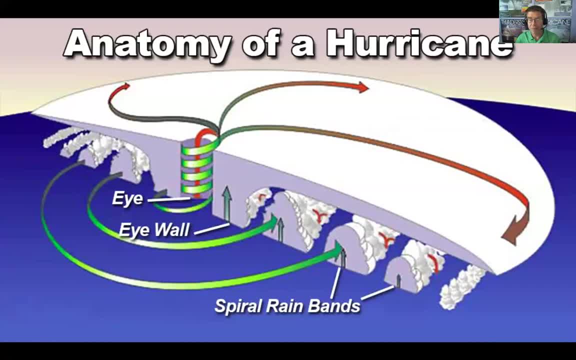 So if I took a big knife and I cut the hurricane in half- and boy it'd have to be a big knife to cut the hurricane in half- you'd see kind of three structures: You'd see the eye, the eye wall and the spiral rain bands. Now, when I'm talking about the eye of the hurricane, 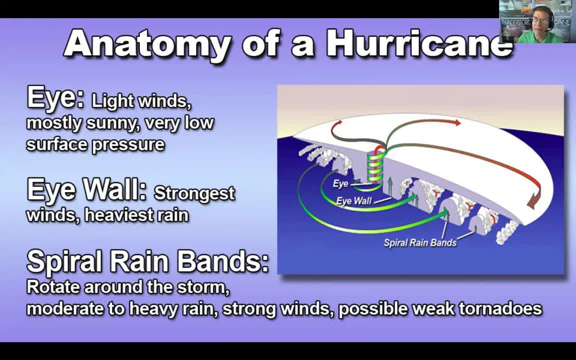 I'm not talking about like an eye like you or I have. The hurricane is not like looking at you or anything like that, It's just the center of the hurricane. Imagine the center point on a pinwheel or the center on a bike's wheel And inside that eye it actually has light. 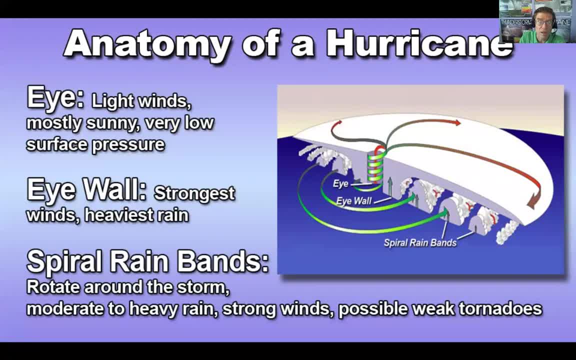 winds and sunny skies, very low surface, Very low pressure, though because it's the middle of that low pressure, It sounds like the eye is the place to be: light winds, mostly sunny, but it's not, because surrounding the eye all the way 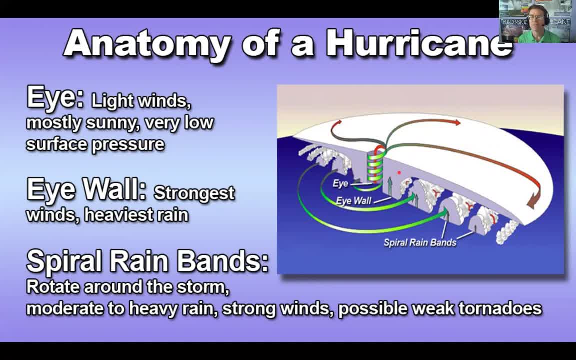 around it is the eye wall. And in the eye wall you've got the strongest winds and the heaviest rains. And radiating out from the eye wall you've got these spiral rain bands. Imagine the arms on a pinwheel or the spokes on a bike wheel And they rotate around the center, that eye of the. 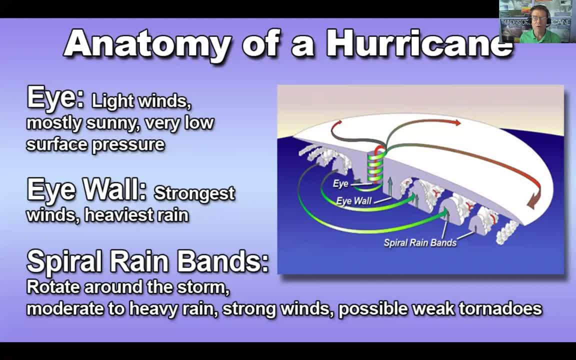 hurricane. And as they rotate, you can get moderate to heavy rain. And as they rotate, you can get moderate to heavy rain. And that's what makes the hurricane such a threat. It has so many different weather threats: Heavy rain, strong winds, weak tornado, storm surge. so many threats. 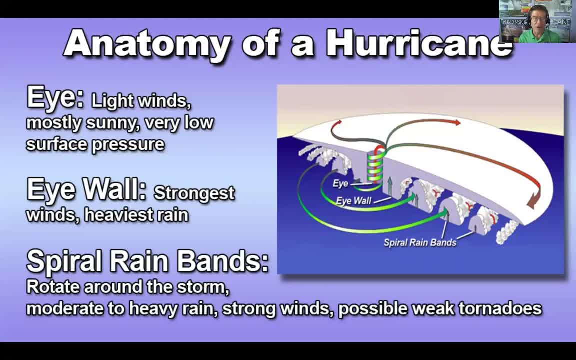 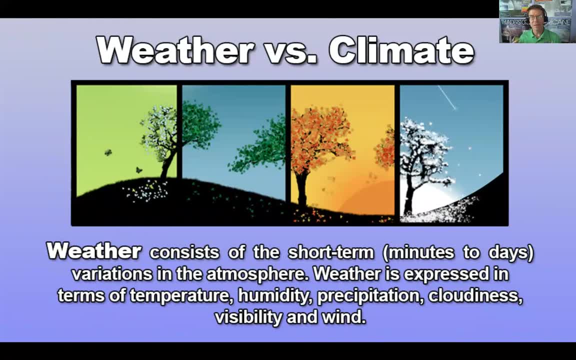 associated with a hurricane And it's so big, it covers such a big area. All right, I'm going to wrap things up with one other section. here We're going to talk about weather versus climate, because a lot of people get these two confused, And it's understandable. they use a lot of the same terms, but they do have a lot of different terms. So I'm going to wrap things up with one real quick one here: Weather versus climate. So I'm going to wrap this up with one real quick one here, And it's something people have been talking about for a long time, But they don't mean quite the 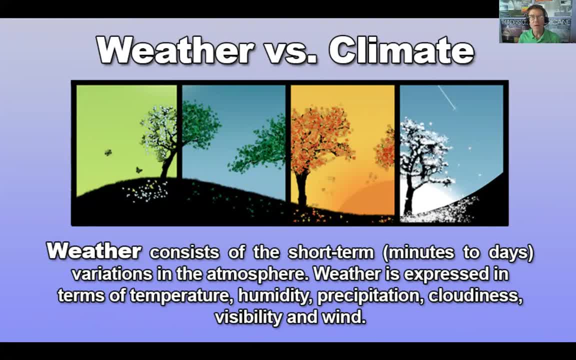 same thing. Weather is talking about the short-term changes in our atmosphere, And when I talk about short-term, I'm going to talk about minutes to days. You guys know the weather can change pretty quickly. If you're sitting at your desk and you look out the window, it's a nice sunny day. you. 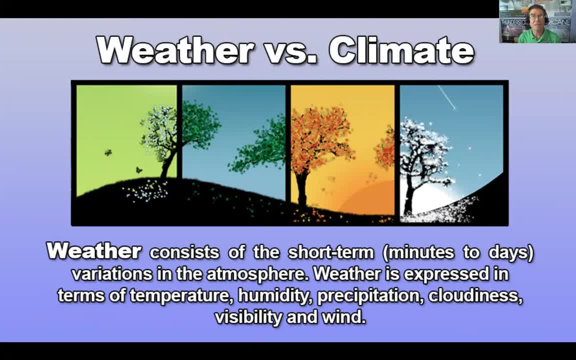 look down to write on something. a few minutes later you look up, the sun's gone. What happened That weather changes very quickly And we use terms like temperature and humidity and precipitation cloudiness when we're talking about weather. So weather is what's going on right now in the 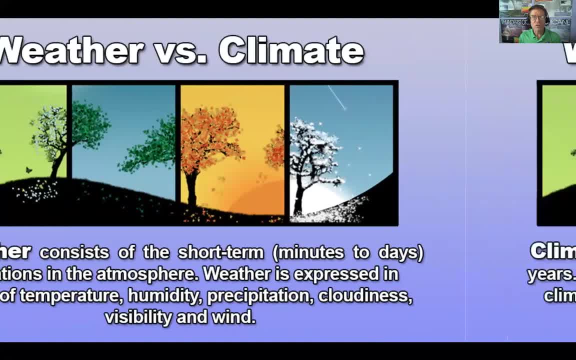 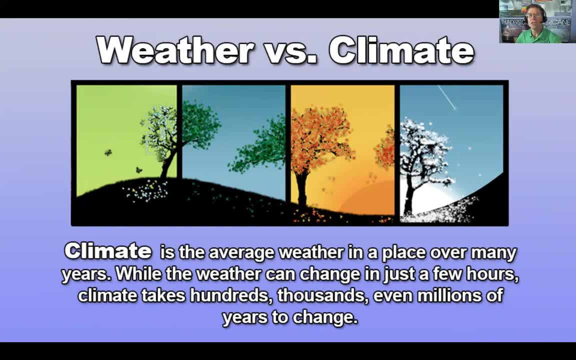 Now what's going on right outside your window is weather versus climate. You know I look at climate as kind of like a math problem. Climate is the average weather in a place over many years. So if you take the average weather, add it all up and divide it by the years, that's how you get the average of something. 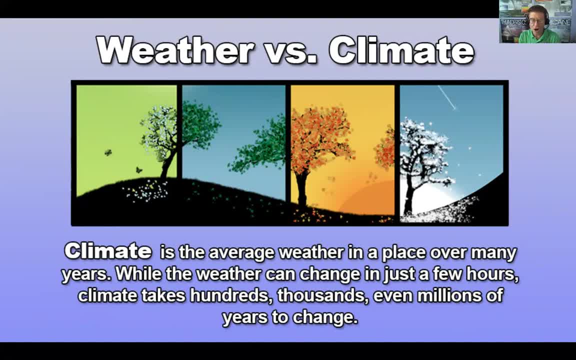 And the climate is the average weather in an area. So if you take all of the summertime temperatures and add them up and then divide by all the days in the summer, you get the average temperature for the summer. And if you multiply- you know, do that over the years- you'll see what the temperature usually is in the summer. 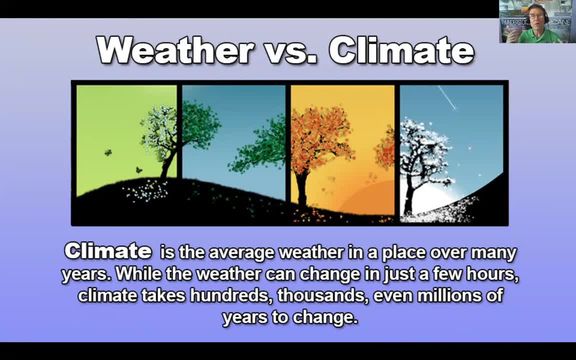 You know, climate is like that average weather over an area And while weather can change in just a few minutes, climate can actually take hundreds or even thousands of years to change Again, because it's that average of the weather in that area. 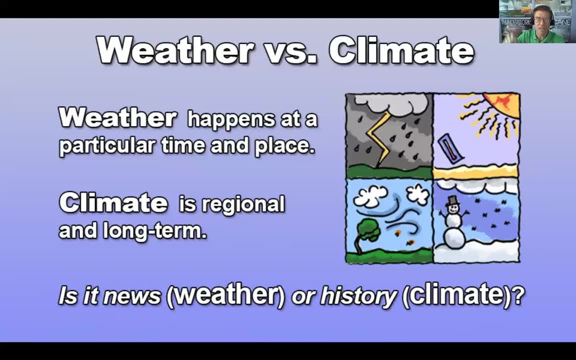 You know, weather is happening at a particular place at a particular time where climate is more regional or long term. You know, I kind of use the example of like the news and history. You know, the news is happening, It's happening right now and it usually is focused in on an area that's happening- like this bank was robbed or something like that- versus history. 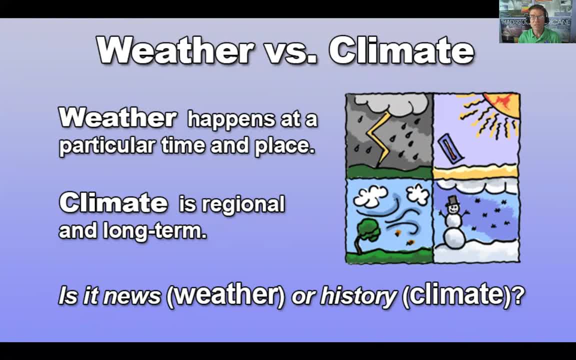 History takes place over a longer time and it usually takes a place over a region. like you know, World War II happened in Europe, kind of thing like that. And those are kind of the two differences, You know. the other example I like to use is: let's say that you live in Jackson Mississippi. 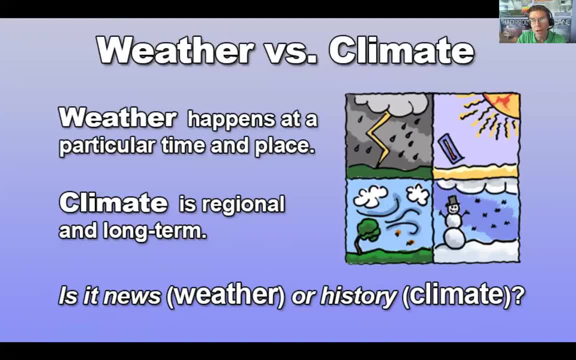 And mom And dad live there with you, but grandma lives in New York City and grandma wants to come visit you during the summer. and they, they say hey, they call you up, say I want to come visit you during the summer. 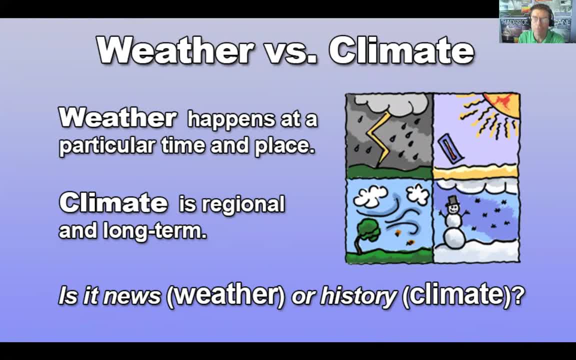 What kind of weather do you get there in Jackson Mississippi during the summer? and you go: oh, grandma, grandma, It can be very hot and sticky in Jackson Mississippi during the summer. So make sure you wear your shorts, your sunglasses and be ready for some hot weather. 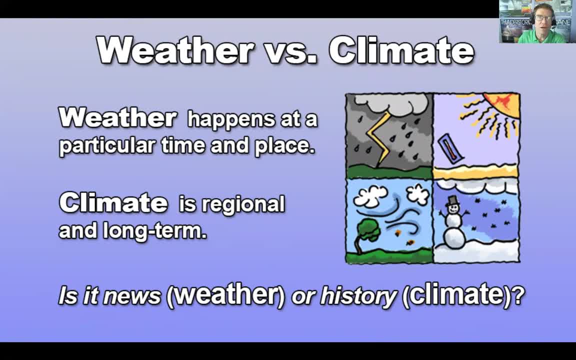 All right. So you The day comes when grandma's going to arrive. She flies in from New York City. You go pick her up at the airport, But on the day she arrives in town it's one of those kind of cool, wet, rainy days. 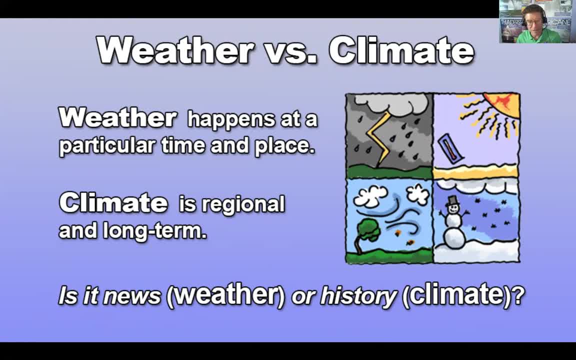 So she comes off the plane, She's got her sunglasses on, She's got her shorts on And she says, hey, you said it's hot and sticky in Mississippi during the summer. And you say, yeah, grandma, that's what it usually is. 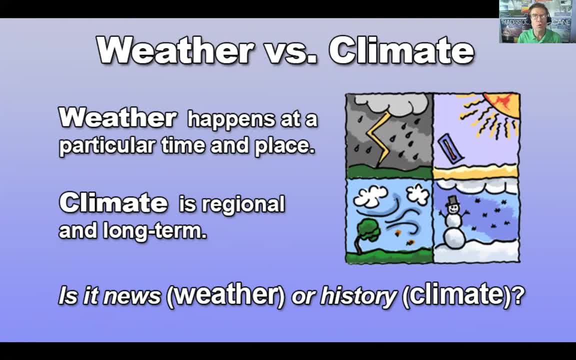 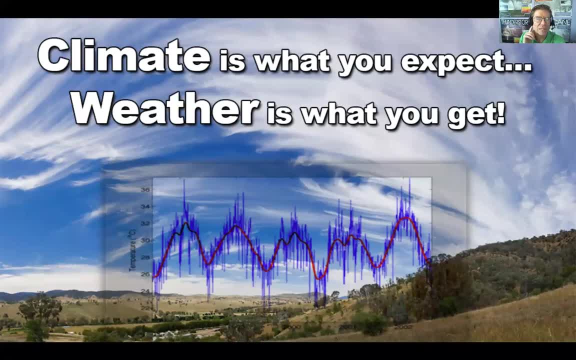 That's the climate. But today it happens to be a cool, wet, rainy day. That's the weather. So that's kind of the differences between the two. You know, we have a saying in the Weather Service: Climate is what you expect, but weather is what you get. 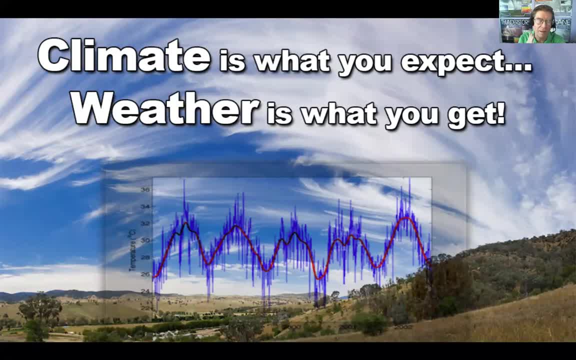 A lot of times in my office I'll get people calling me in like March and saying, hey, we're going to do a June wedding. What's the weather going to be in June? I say I can't tell you what the weather is going to be in June. 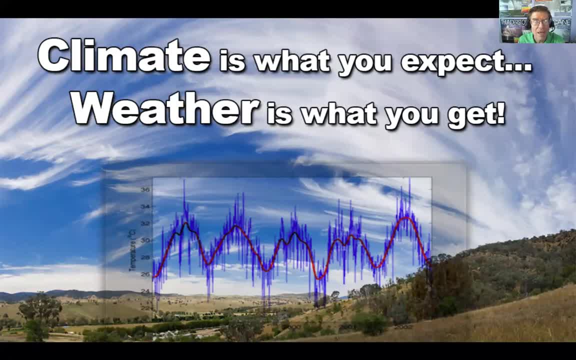 I can't forecast that far out, But I can tell you what the climate is, And the climate in June in El Paso is hot and dry. Does that mean that on the day of the wedding, when it comes to June, that it will be hot and dry? 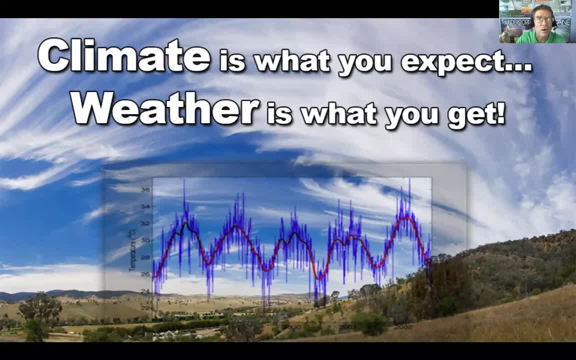 There's a good chance that it will be, but not necessarily. It could be one of those rare days when it actually is a cool, wet, rainy day. So again, climate is what you expect, but weather is actually what's going on when you look outside that window. 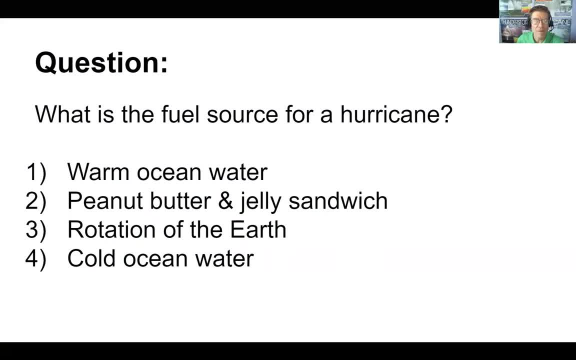 All right, I got a few more questions for you and then we'll wrap things up All right. So what is the fuel source for a hurricane? Is it one warm ocean water, Two peanut butter and jelly sandwich- My favorite. 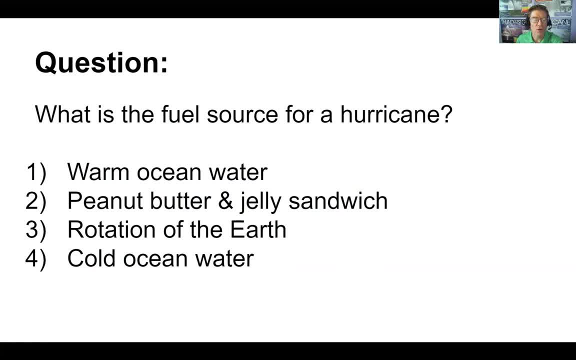 Three, Four- the rotation of the earth- Or four cold ocean waters. What do you guys think? I don't know how many of you all said peanut butter and jelly sandwich. I know I was thinking about it, but it's actually those warm ocean waters. 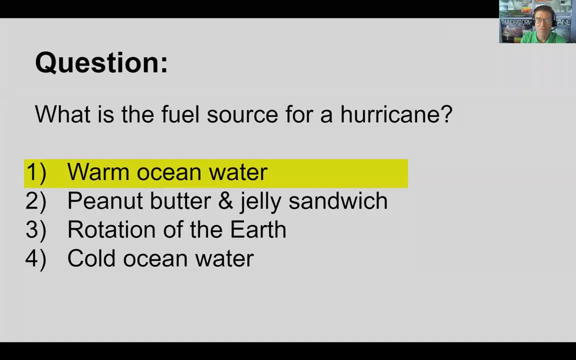 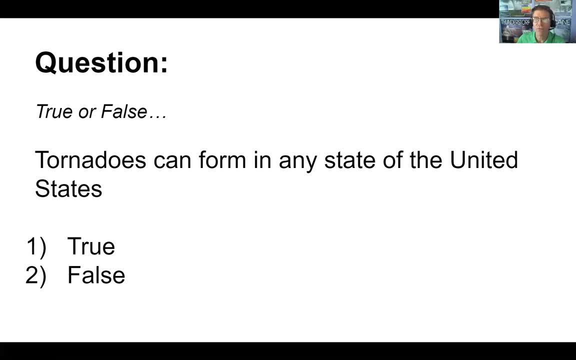 That's what fuels those hurricanes. All right. Question number two: Oh yay, True or false, Tornadoes can form in any state of the United States. Is that true or false? You remember that map that I put up there? 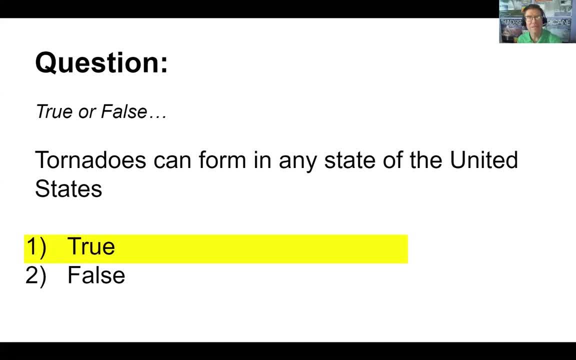 I hope you remember that. Yes, tornadoes can form in any state of the United States. They're just most likely to form kind of in the middle part of the United States, what we call Tornado Alley. And I think I've got one more question here.